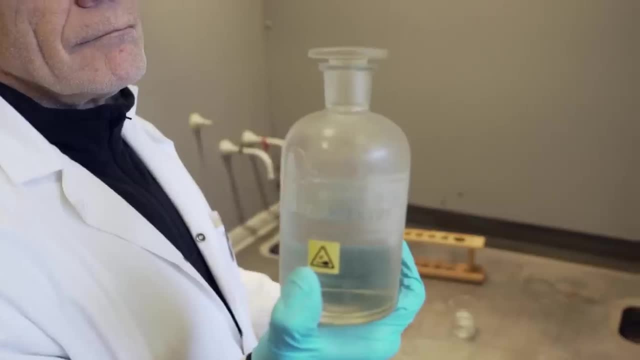 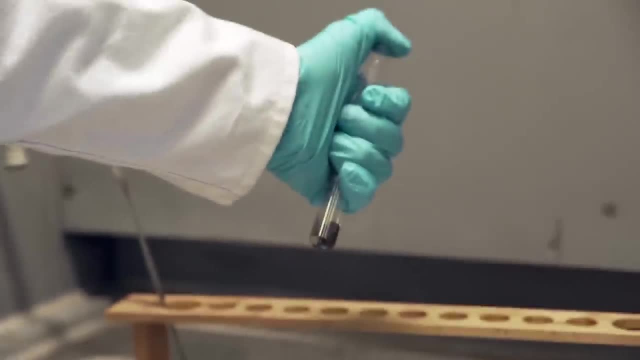 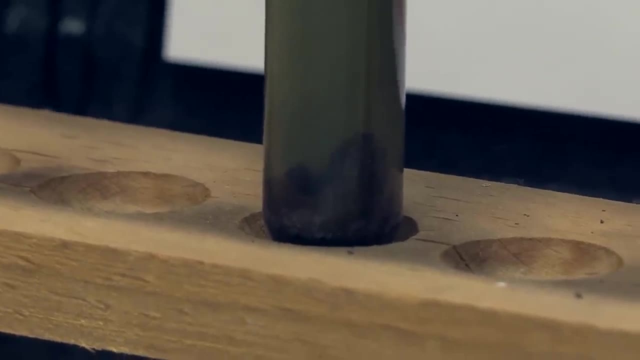 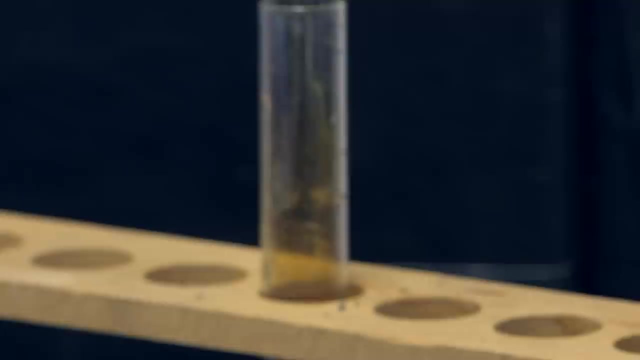 At this stage hold and Shravira continues. There's quite a violent reaction, Lots of bubbling, and it forms the gas NO nitric oxide, which is colourless, but it reacts with air to give nitrogen dioxide, which is brown, So you can see brownish fumes coming out of the test tube. 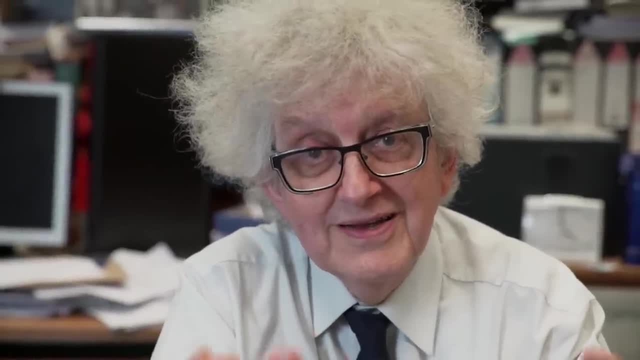 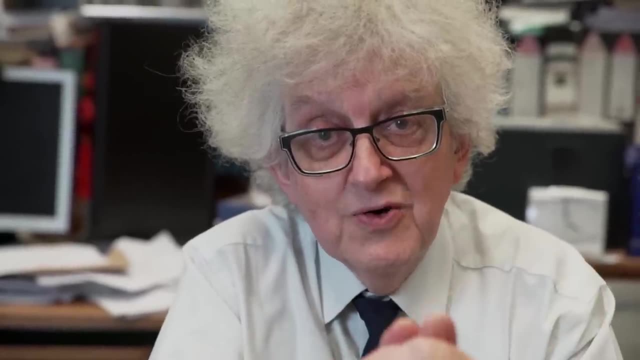 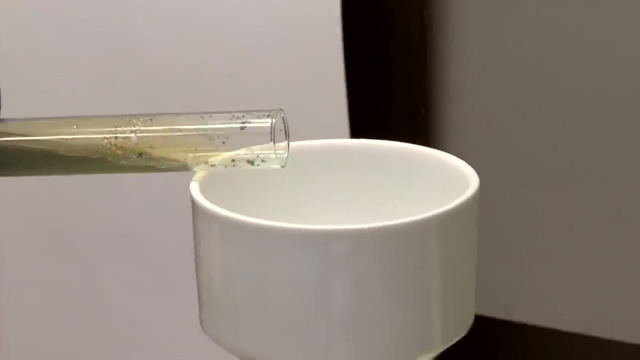 The textbooks say that when you dissolve arsenic In nitric acid you make a solution of the oxide. we want the poisonous oxide. It's meant to taste of sugar. Neil set up a very nice filter system, poured the solution in and it came through. 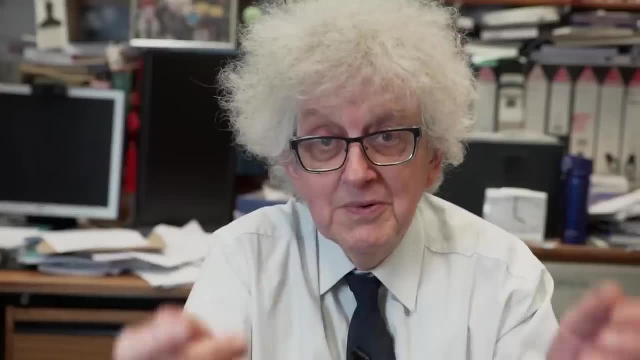 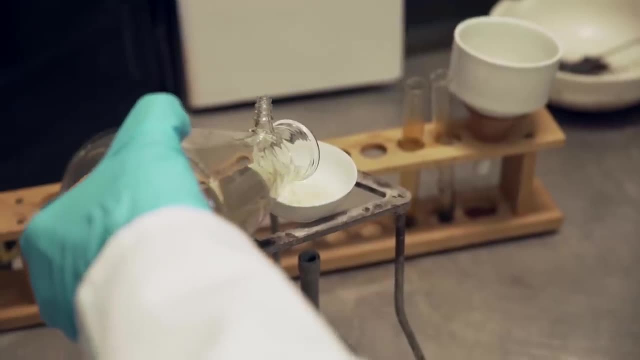 Though I must say it did still look a little brown, But we were really hopeful We were going to get our white powder. The next stage, of course, is to go from solution to solid, So you have to evaporate off the water. 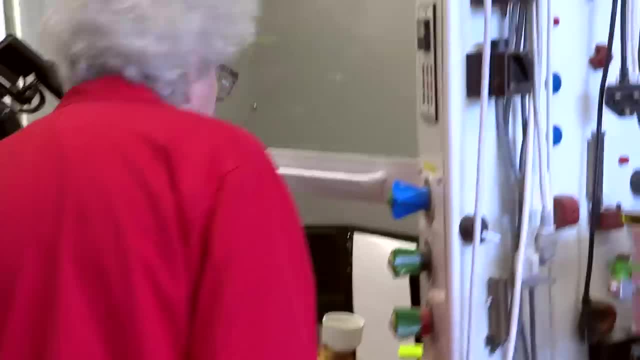 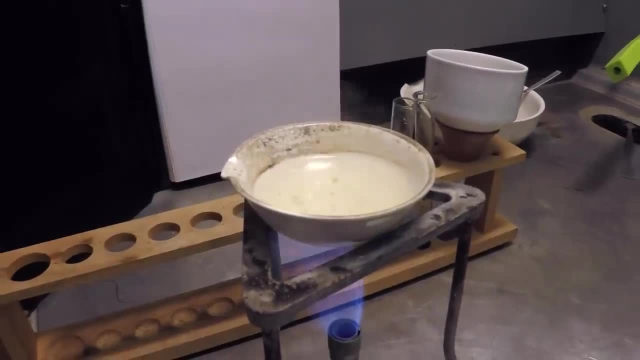 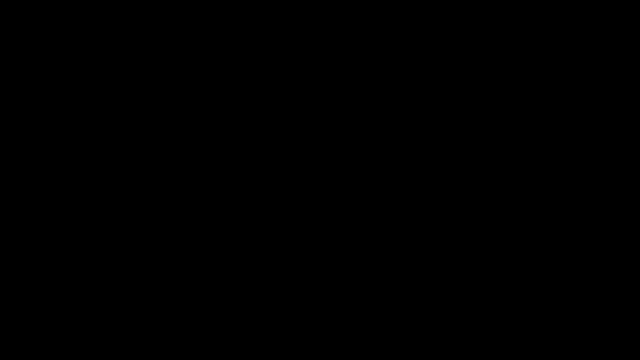 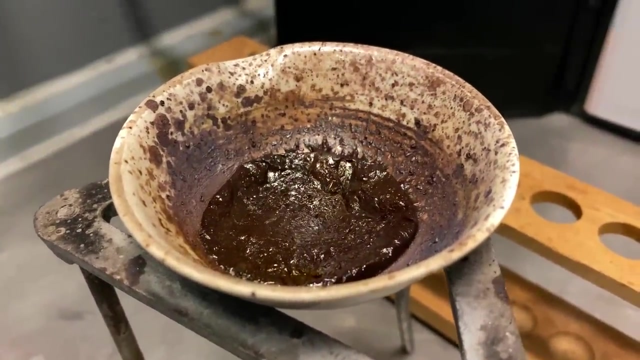 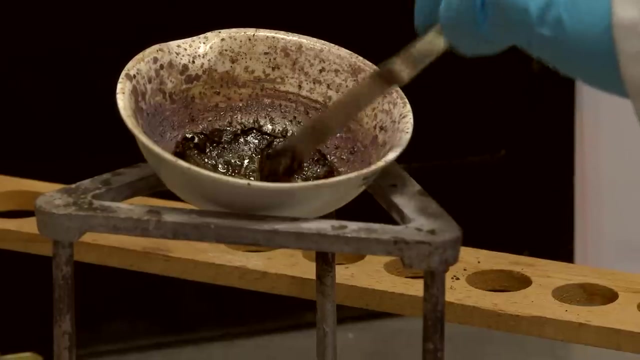 It was a bit slow process. I got bored and went out while Neil was finishing it. That's pure failure. What a disappointment. Instead of this lovely white powder, there was some sticky brown solid, I presume because we've still got some particles of arsenic. 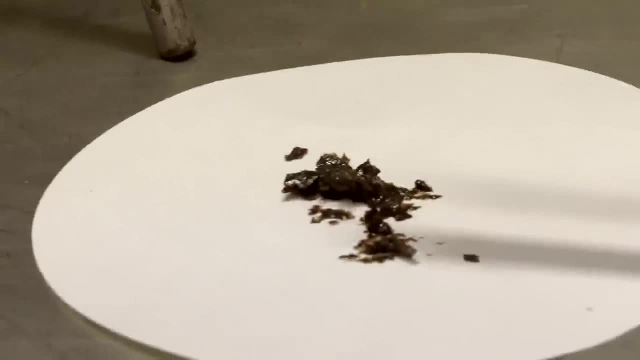 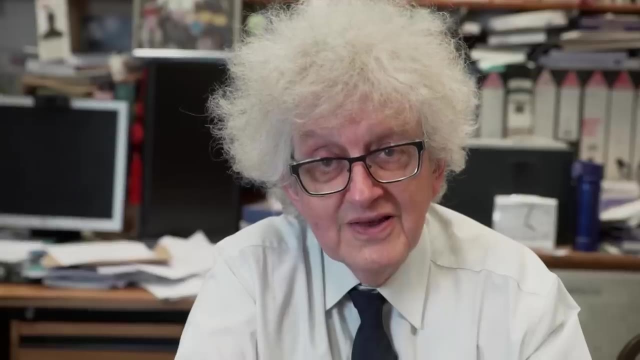 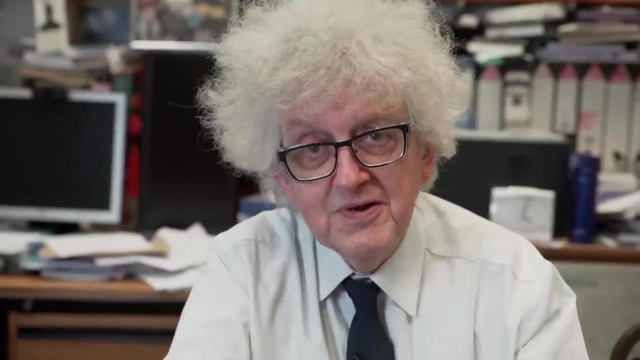 in the white powder- at least we tried, But I still think it's probably arsenic oxide. The reason they used arsenic oxide was they could easily get it. It was a white powder. it tasted sweet, so it wasn't very noticeable if you mixed it with sugar. 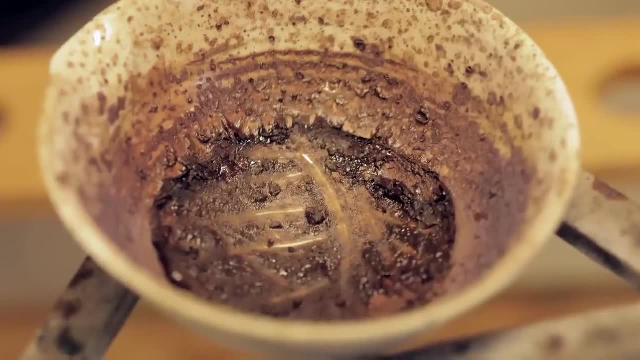 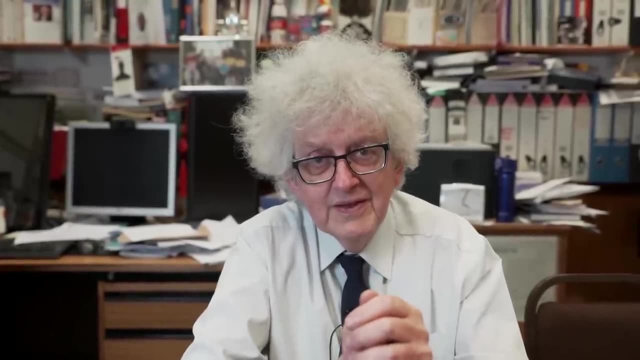 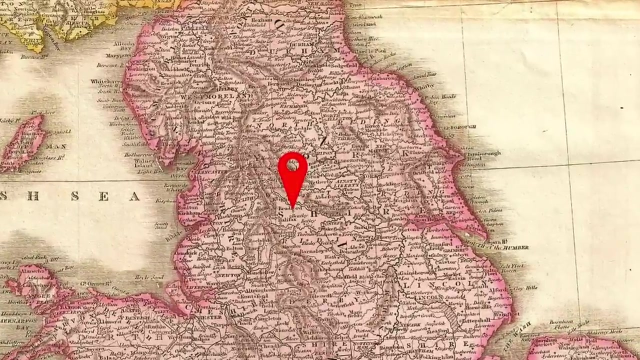 So our brown stuff is not going to be much use for poisoning people. Fortunately, we're not going to try. I have two favorite stories about poisoning. Both of them are true. The first one happened in a town in the north of England called Bradford. 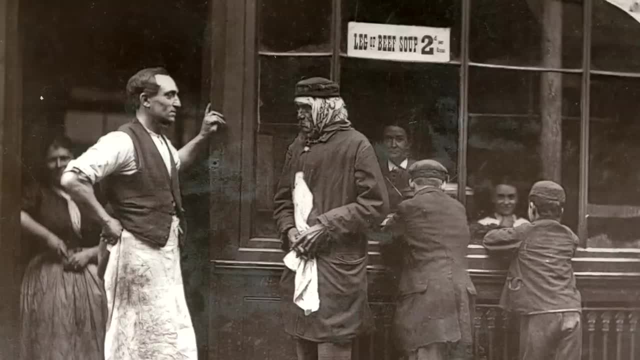 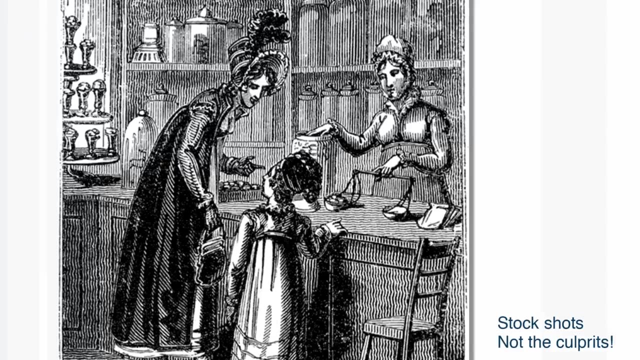 It happened in 1858 in October. In those days sugar was quite expensive, So people who made sweets were very dishonest and added some cheap powder To the sugar so that they didn't have to put so much sugar in the sweets. 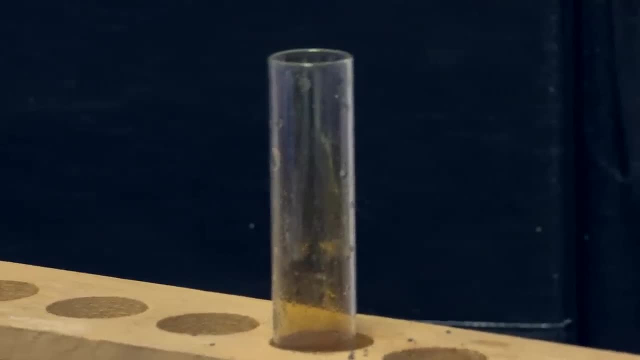 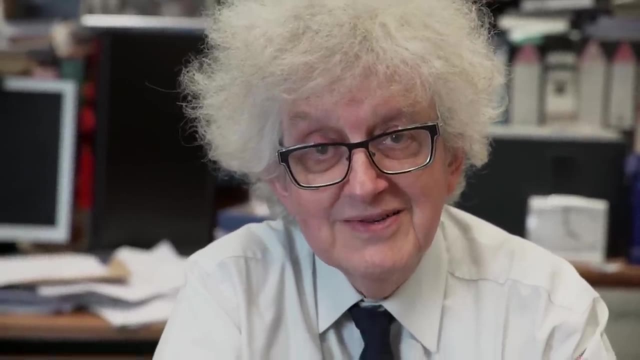 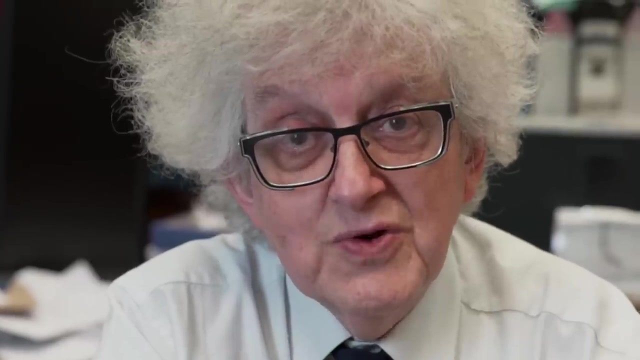 So you can see brownish fumes coming out of the test tube. The textbooks say that when you dissolve arsenic in nitric acid you make a solution of the oxide. we want the poisonous oxide. It's meant to taste of sugar. Neil set up a very nice filter system, poured the 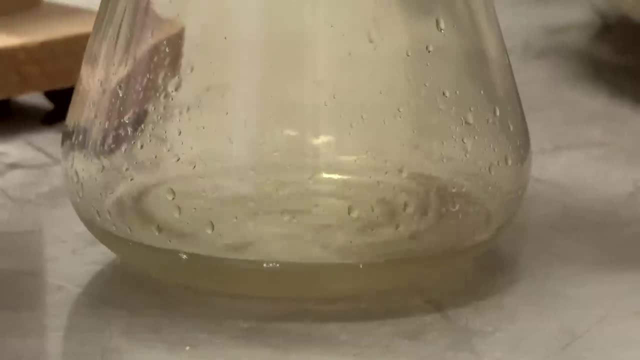 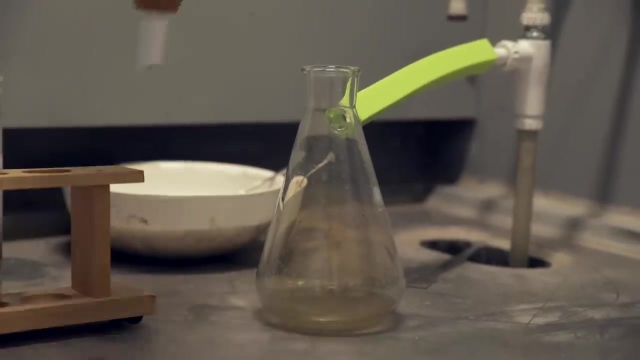 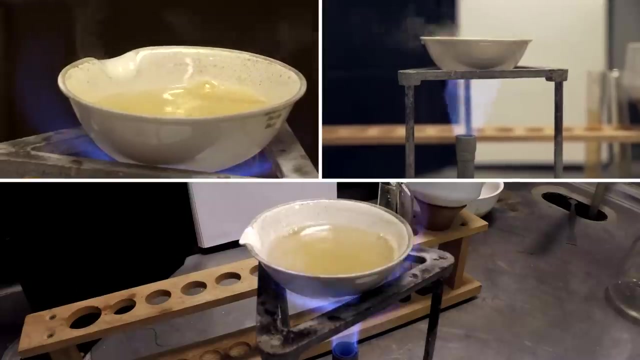 solution in and it came through, Though I must say it did still look a little brown, But we were really hopeful we were going to get our white powder. The next stage, of course, is to go from a solution to a solid, so you have to evaporate. 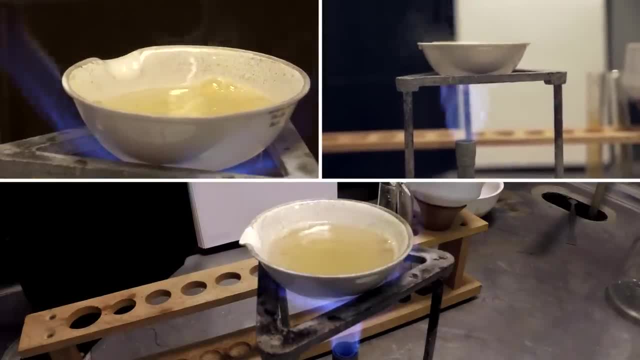 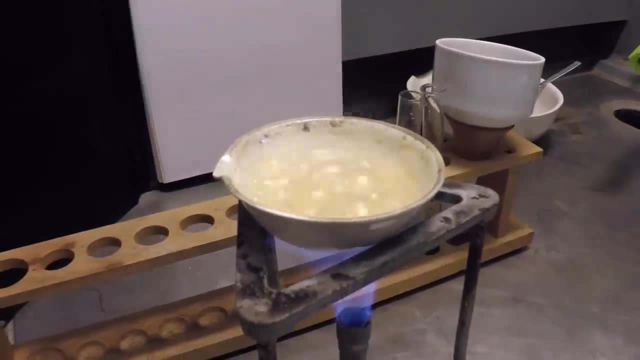 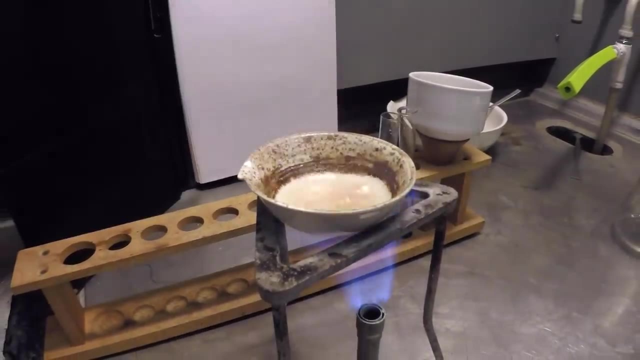 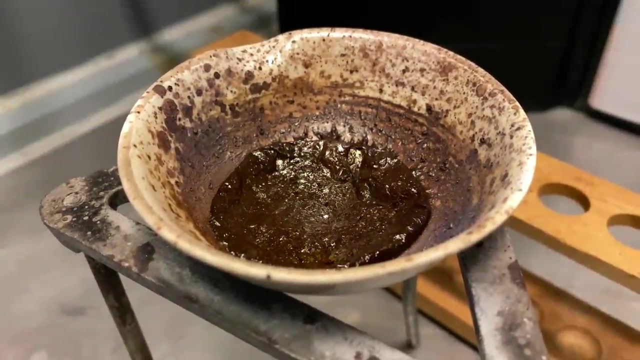 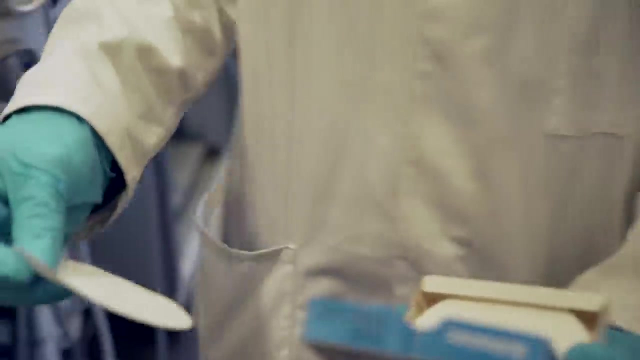 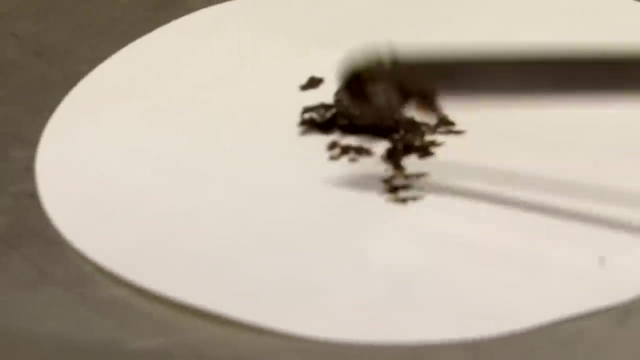 off the water. It was a bit slow process. I got bored and went out while Neil was finishing it. That's pure failure. What a disappointment. Instead of this lovely white powder, there was some sticky brown solid, I presume because we've still got some particles of arsenic in the white powder. 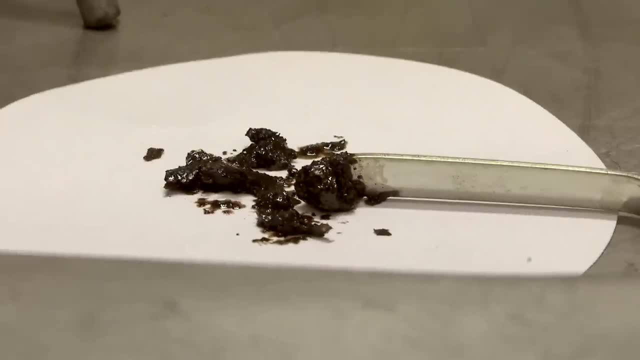 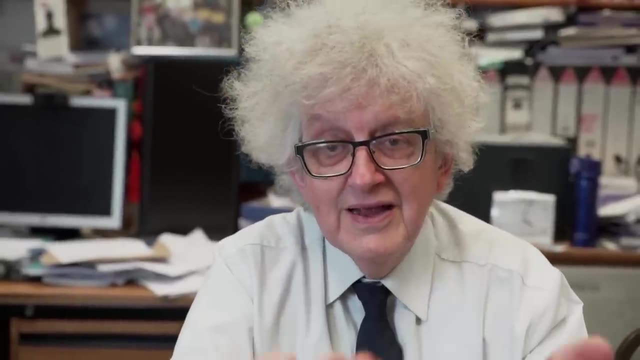 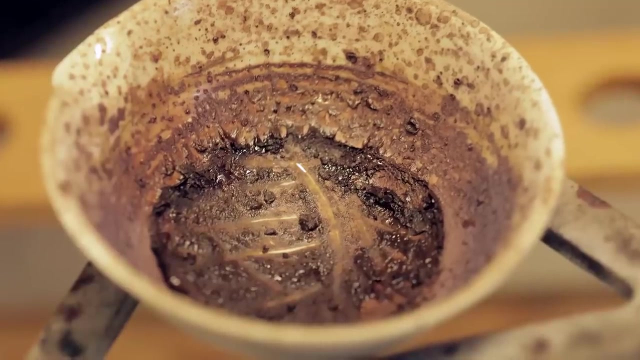 at least we tried, But I still think it's probably arsenic oxide. The reason they used arsenic oxide was they could easily get it. It was a white powder. it tasted sweet so it wasn't very noticeable if you mixed it with sugar. So our brown stuff is not going. 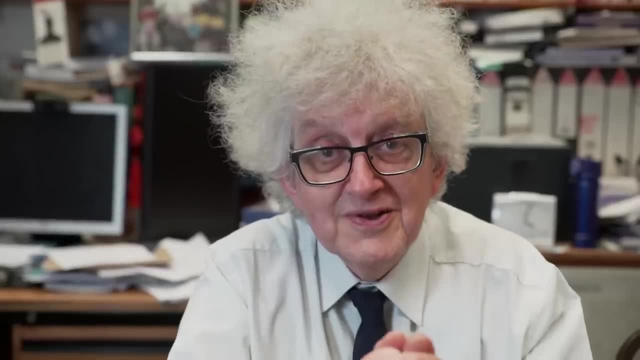 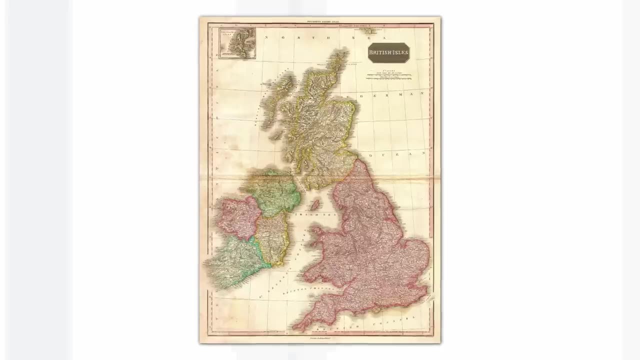 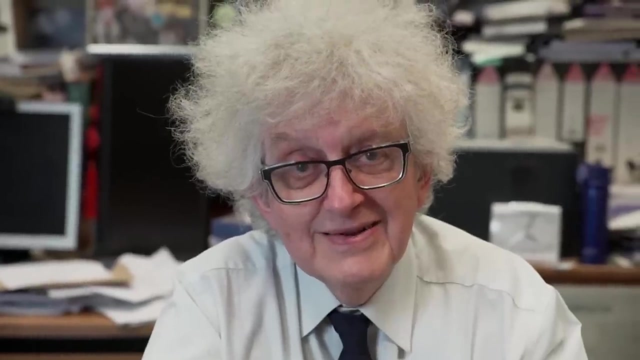 to be much use for poisoning people. Fortunately we're not going to try. I have two favorite stories about poisoning. Both of them are true. The first one happened in a town in the north of England called Bradford. It happened in 1858, in October. In those days. 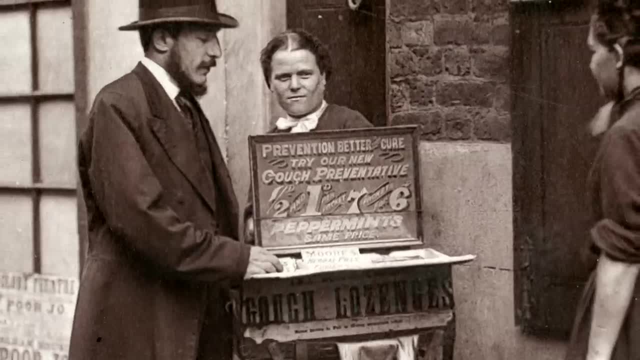 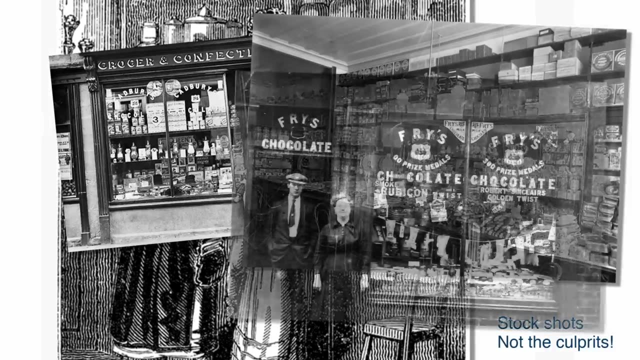 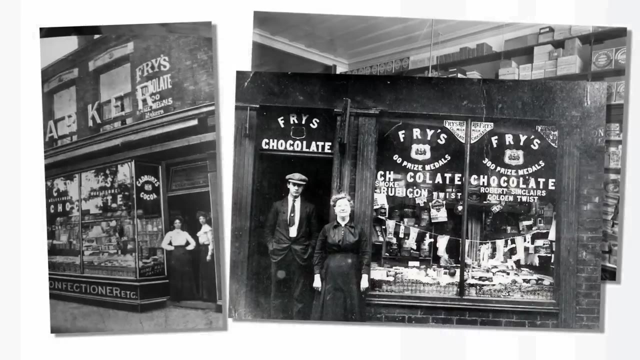 sugar was quite expensive. What, What Well, the people who were making the sweets were very dishonest and added some cheap powder to the sugar so that they didn't have to put so much sugar in the sweets. They called this white powder daft. On this particular occasion, a sweet maker called John Neil sent his lodger. 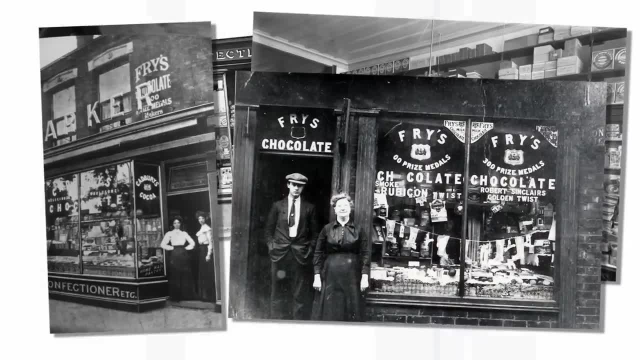 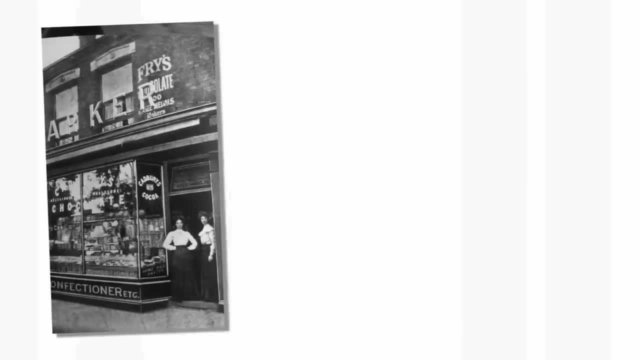 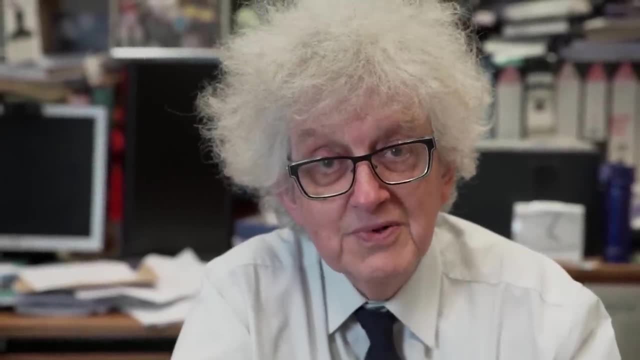 They called this white powder daft. On this particular occasion, a sweet maker called John Neal sent his lodger to go and get some daft to put in his next batch of sweets. He called them lozenges And he went to the next town. 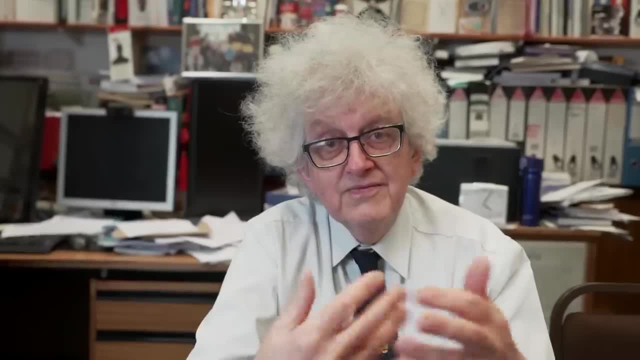 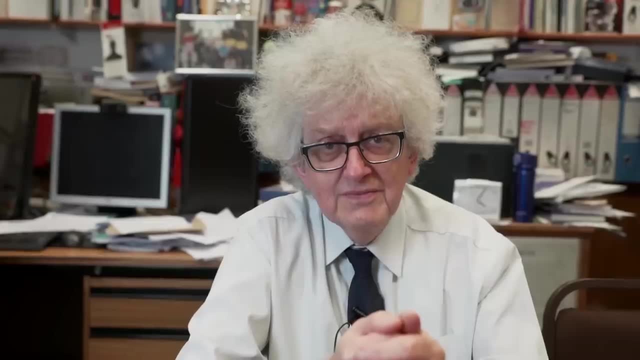 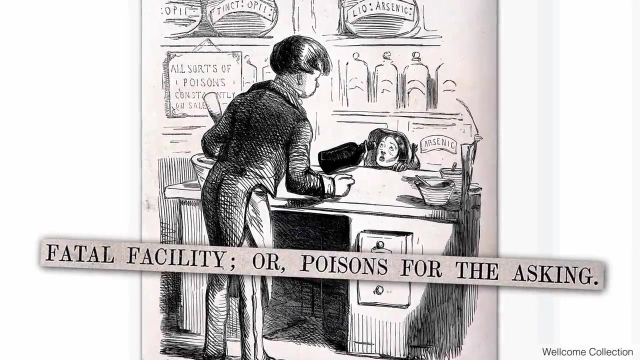 and went to a pharmacist and the pharmacist told his assistant to go and fetch the daft, which was a white powder, And unfortunately he didn't explain correctly, So the pharmacist sold 12 pounds, that's five kilos of arsenic oxide, to the unfortunate customer. 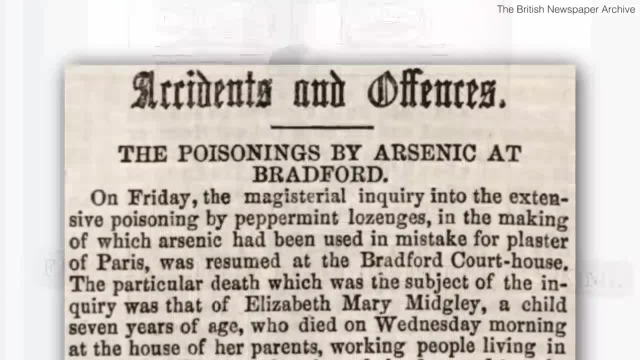 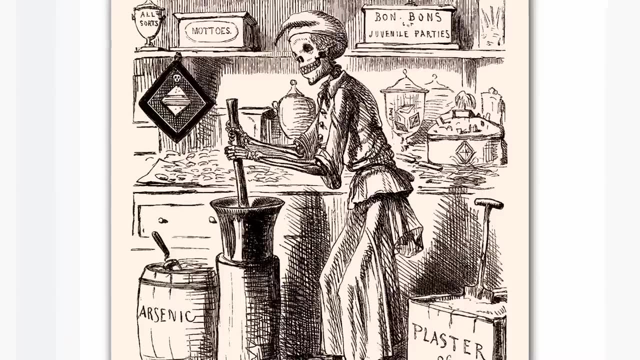 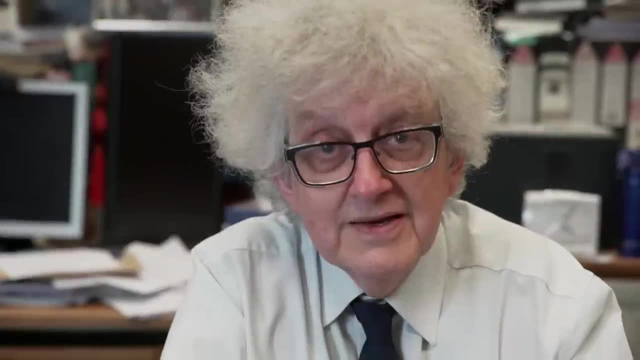 This was mixed in with a sweet mixture and more than 20 people died of arsenic poisoning in Bradford and more than 200 were really ill, And this was one of the things that led to a greater control of arsenic in the United Kingdom. 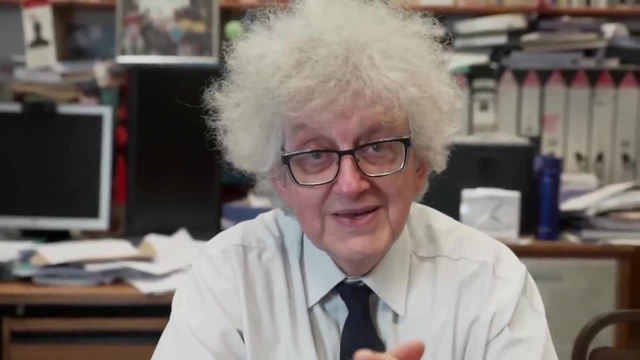 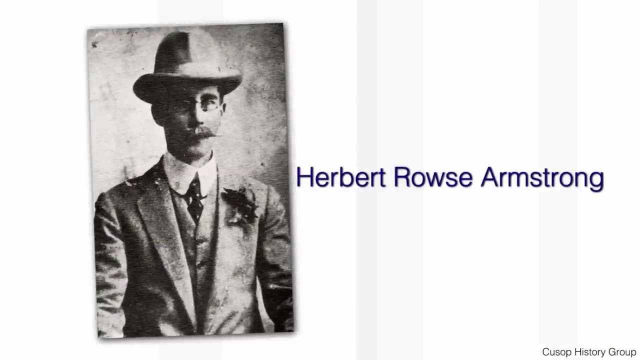 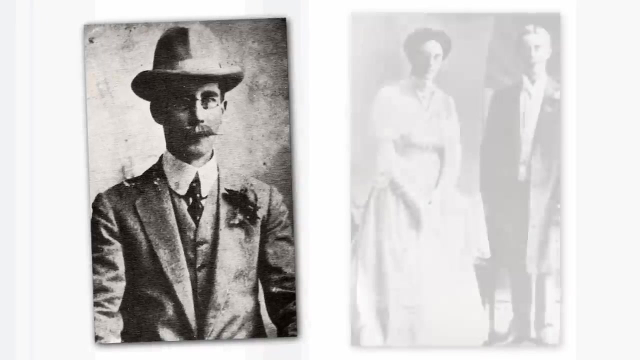 The other case took place in the early 1920s in a town in the west of England called Hay-on-Wye. The attacks were carried out by a solicitor, a lawyer, who, in fact, was the only lawyer who's ever been hanged in the UK. 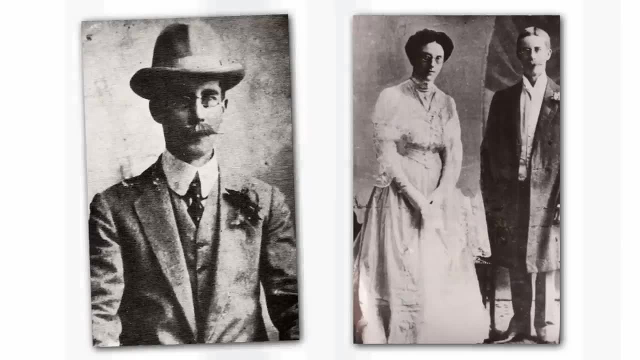 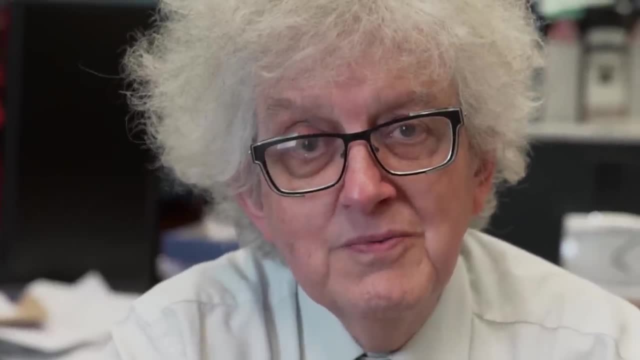 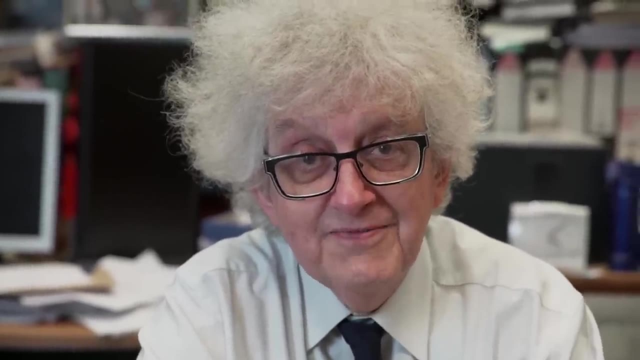 It is believed he poisoned his wife with arsenic over a period of several months, And then one of his business rivals was invited to tea. The lawyer passed a scone, a little cake in his fingers, to his rival, And as he passed it he said: 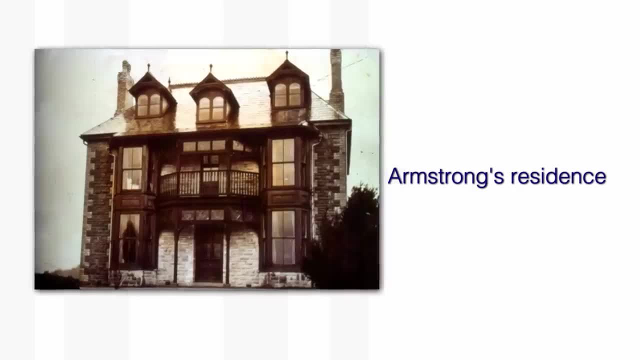 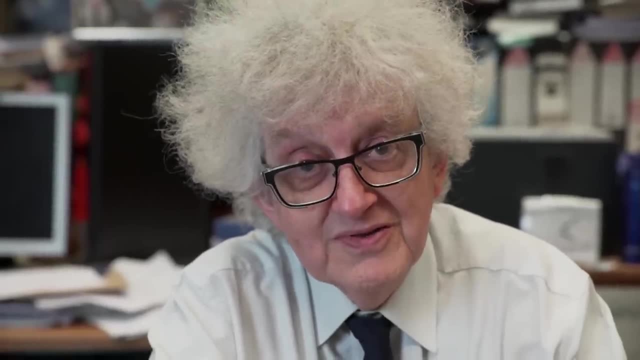 excuse fingers And in that moment, it is believed he put arsenic on the cake. His guest was very ill and was found to have been poisoned with arsenic, So they exhumed the body of his wife, dug it up and it was full of arsenic. 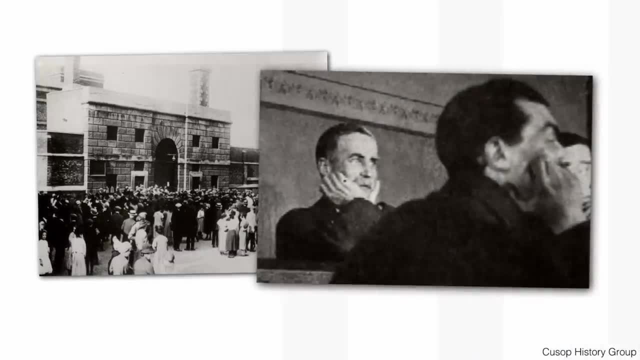 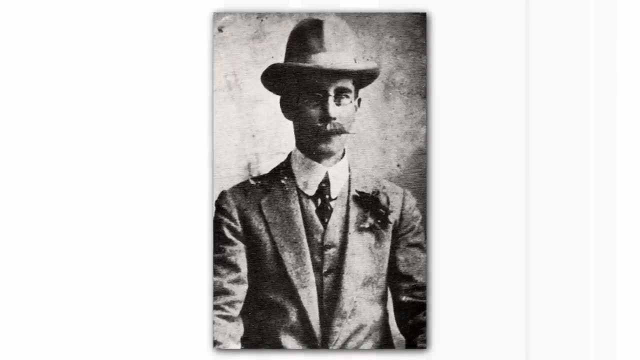 So he was tried and convicted and was executed, And it should be said that he always denied that he had done this. though, when he was arrested, he did have arsenic powder in a packet in his pocket. Did he have good white powder or brown sludge? 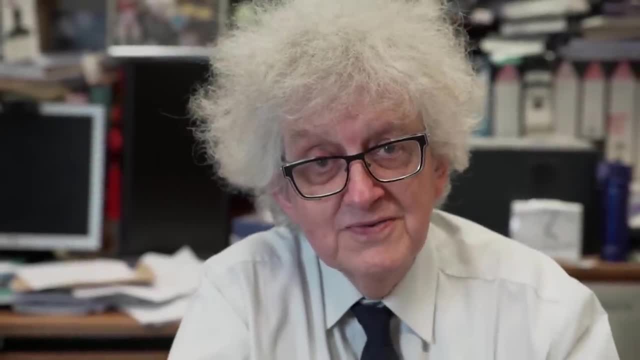 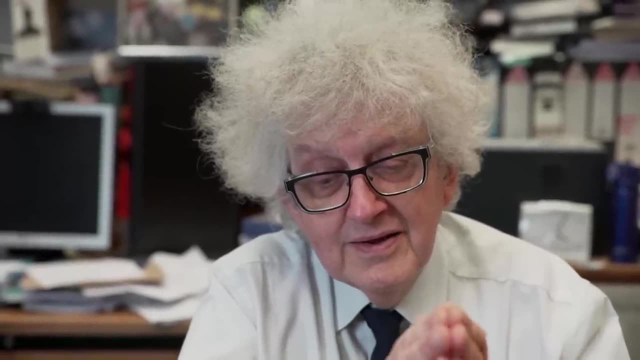 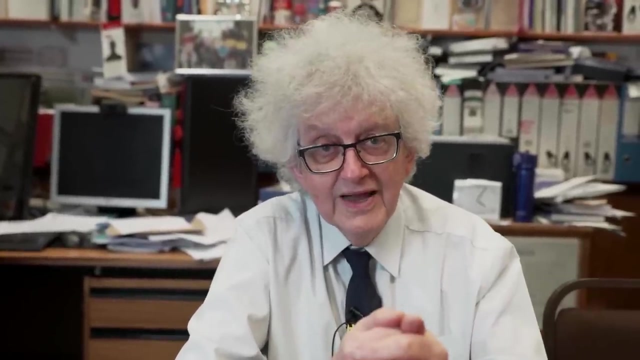 to go and get some daft to put in his next batch of sweets. He called them lozenges- And he went to the next town, went to a pharmacist and the pharmacist told his assistant to go and fetch the daft, which was a white powder, and unfortunately he didn't explain. 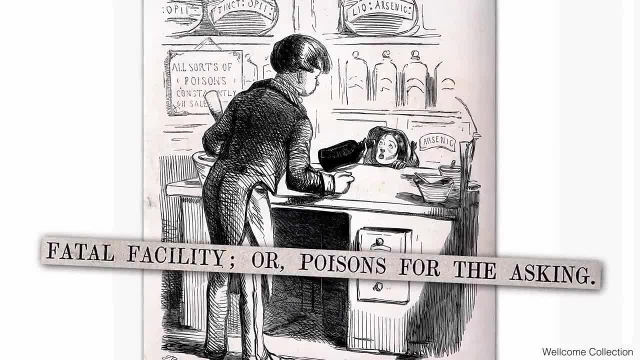 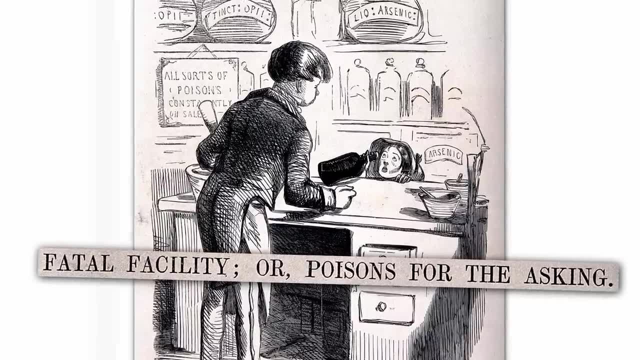 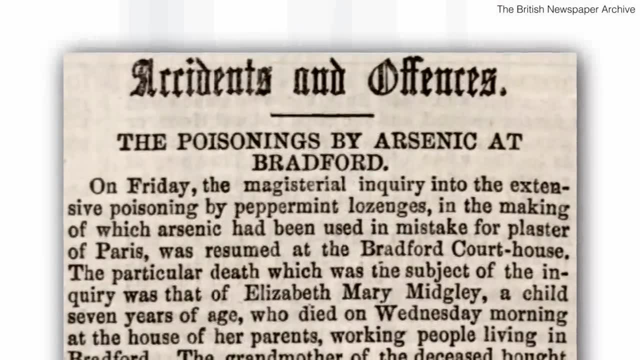 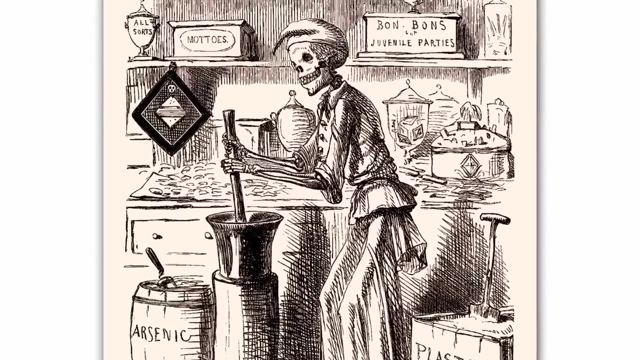 correctly so the pharmacist sold 12 pounds, that's five kilos of arsenic oxide, to the unfortunate customer. this was mixed in with a sweet mixture and more than 20 people died of arsenic poisoning in Bradford and more than 200 were really ill, and this was one of the things that led to a greater control of. 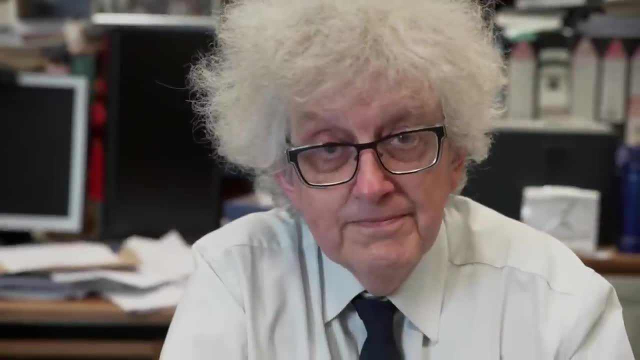 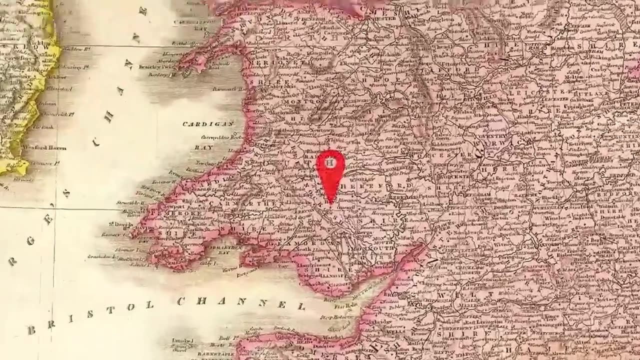 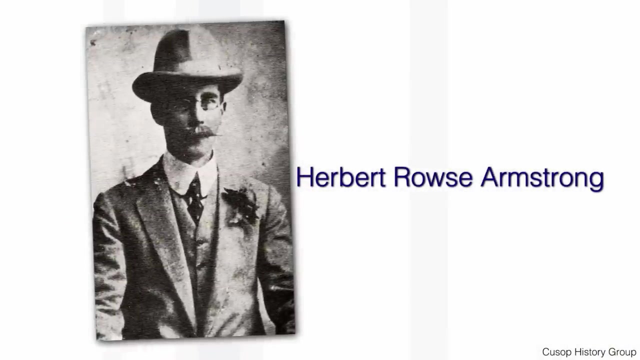 arsenic in the United Kingdom. the other case took place in the early 1920s in a town in the west of England called Hay, on why the attacks were carried out by a solicitor, a lawyer who in fact was the only lawyer who's ever been hanged in the UK. it is believed he 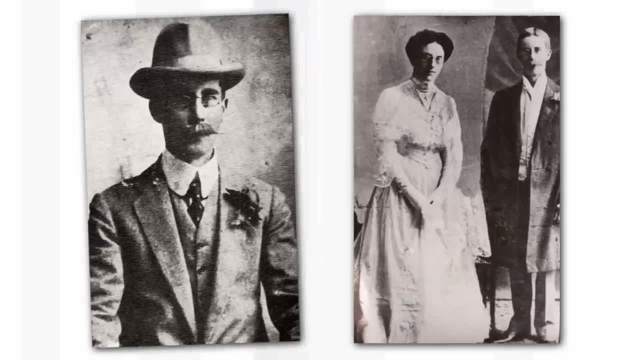 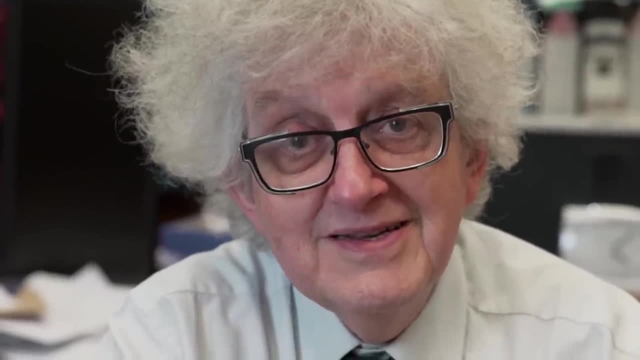 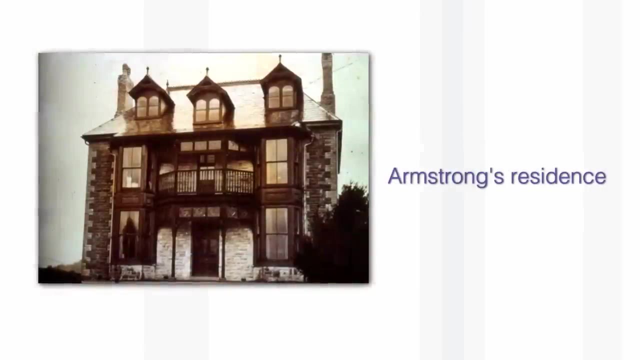 poisoned his wife with arsenic over a period of several months, and then one of his business rivals was invited to tea. the lawyer passed a scone, a little cake in his fingers, to his rival and as he passed it he said: excuse fingers. and in that moment 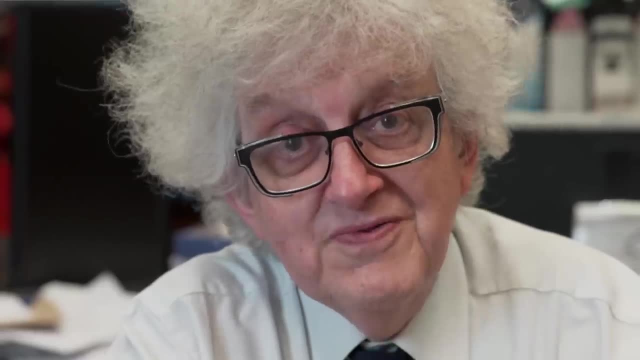 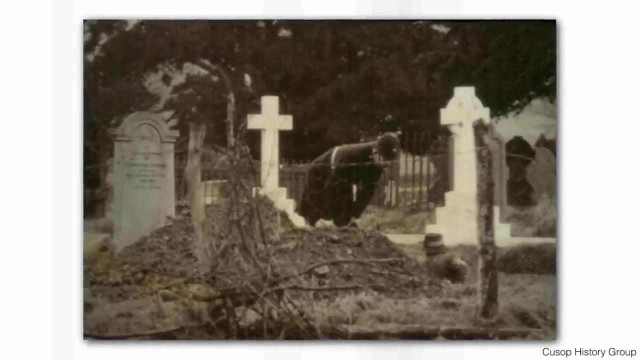 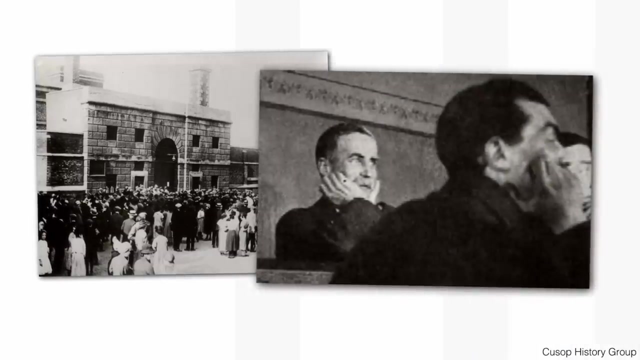 it is believed, put arsenic on the cake. His guest was very ill and was found to have been poisoned with arsenic, so they exhumed the body of his wife, dug it up and it was full of arsenic. So he was tried and convicted and was executed. 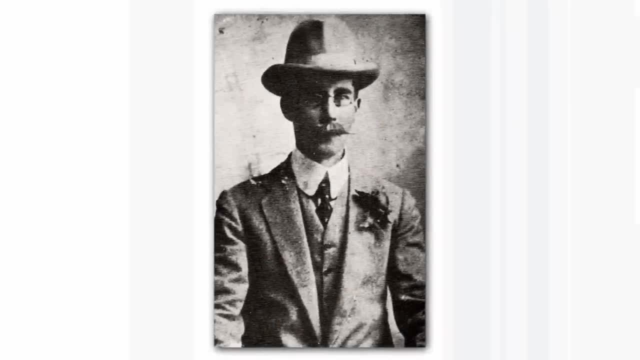 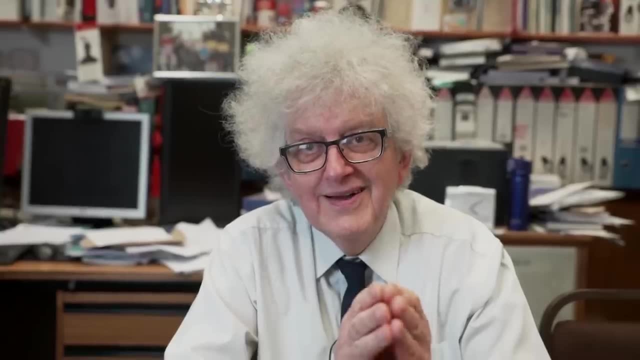 And it should be said that he always denied that he had done this. though when he was arrested he did have arsenic powder in a packet in his pocket. Did he have good white powder or brown sludge? He had nice white powder. 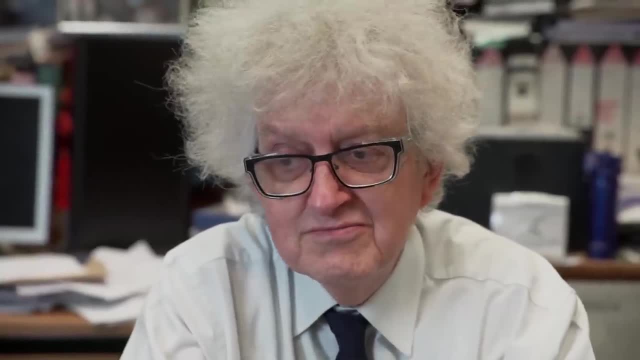 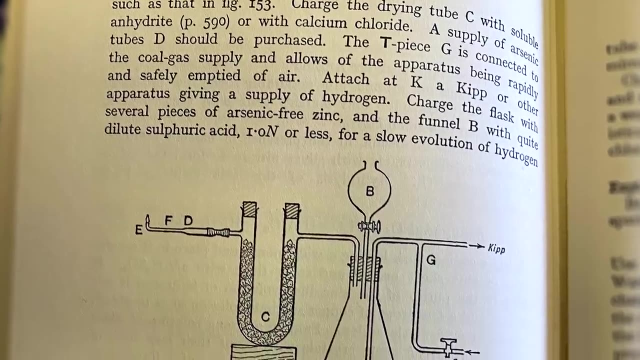 The question is, how did they find arsenic in the body of his dead wife, who'd been under the ground for several months? And it's with a very clever test that was invented in the early 19th century called Marsh's Test. 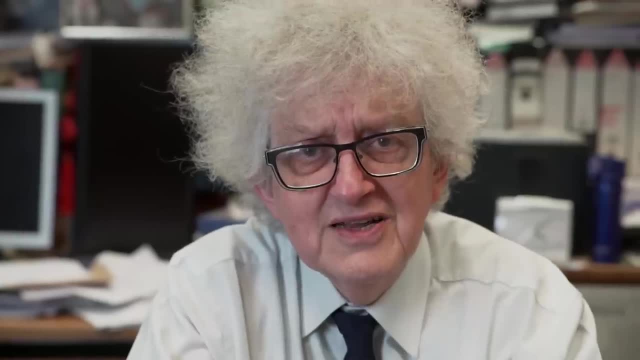 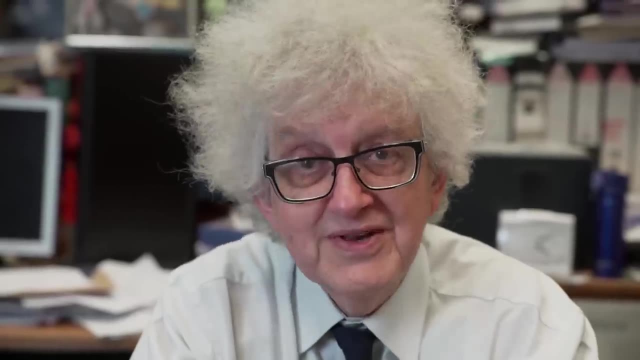 He had nice white powder. The question is, how did they find arsenic in the body of his dead wife, who'd been under the ground for several months, And it's with a very clever test that was invented in the early 19th century. 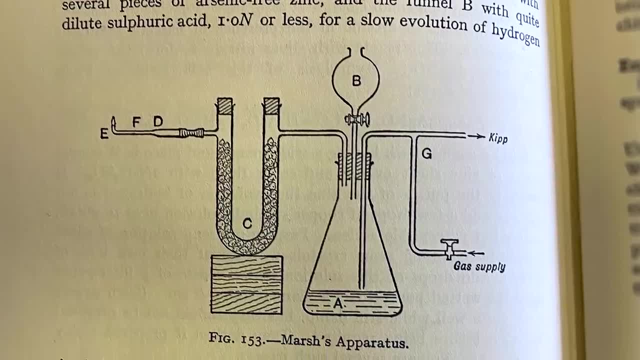 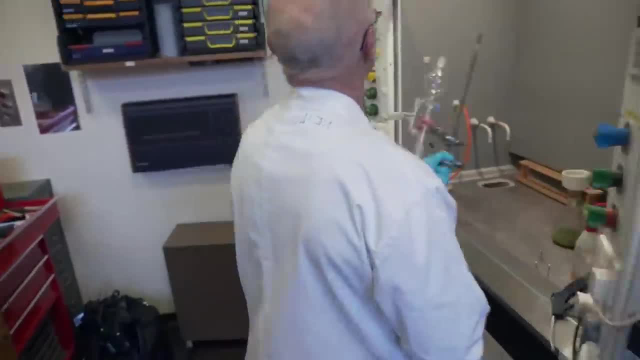 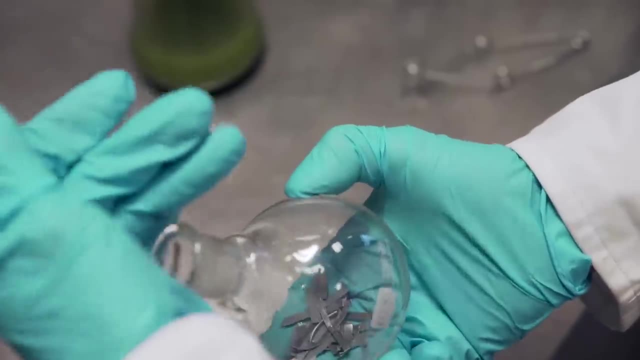 called Marsh's test And Neil decided he would like to do Marsh's test too. The first thing you have to do is to add metallic zinc. I was really excited I was allowed to chop up the zinc. You put in the pieces of zinc into a round bottom flask. 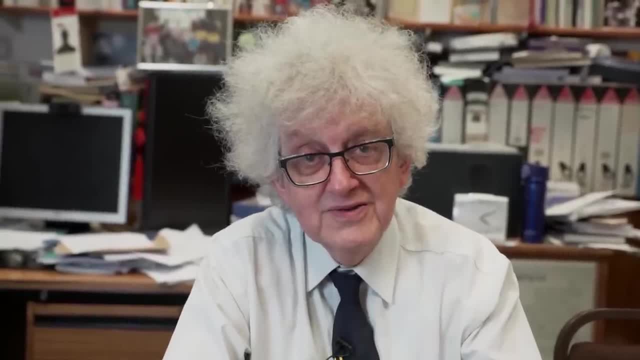 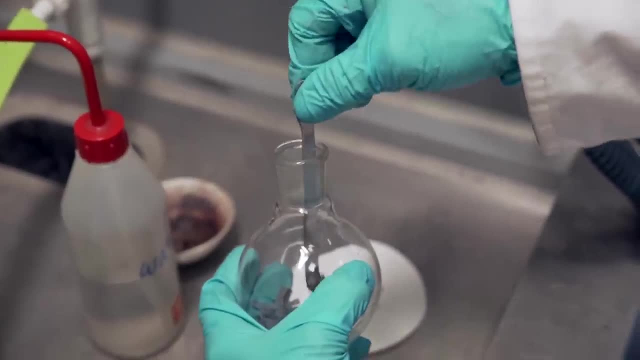 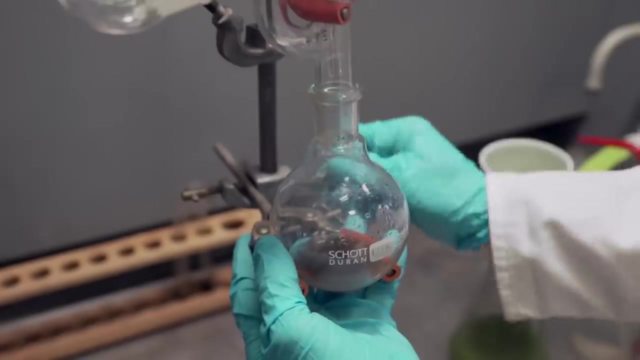 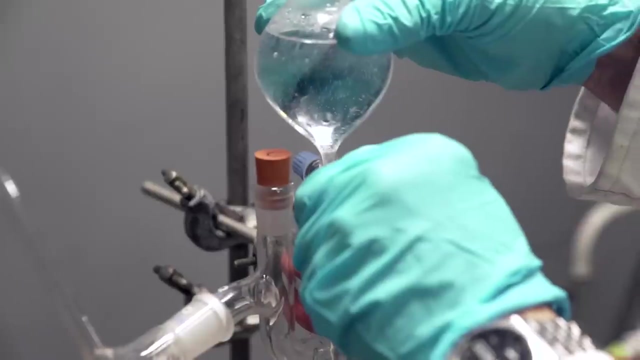 and then you add whatever you think contains arsenic, In our case a small amount of Neil's brown sludge. And then from a dropping funnel you drop in dilute sulfuric acid, and the sulfuric acid reacts with the zinc. 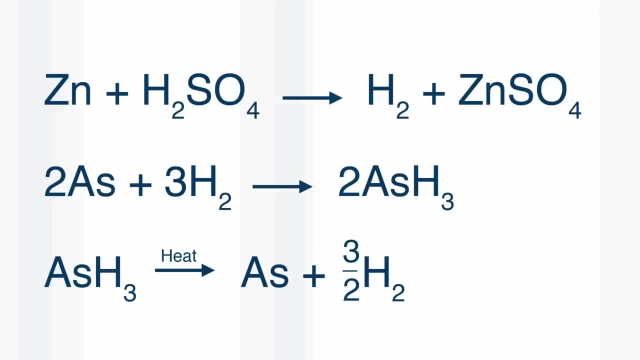 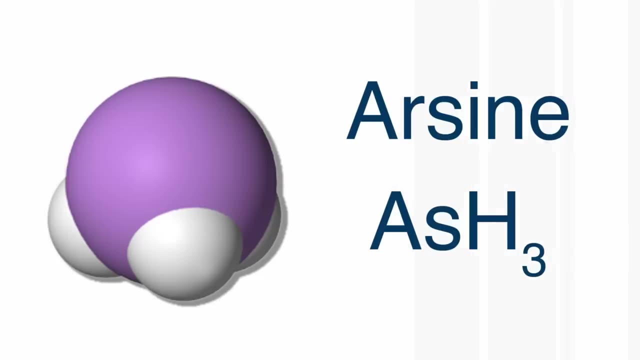 and generates hydrogen. And the hydrogen reacts with the arsenic and makes a compound which has a similar formula to ammonia, but it has three hydrogens attached to arsenic rather than three hydrogens attached to nitrogen, which you have in ammonia, And this compound called arsine. 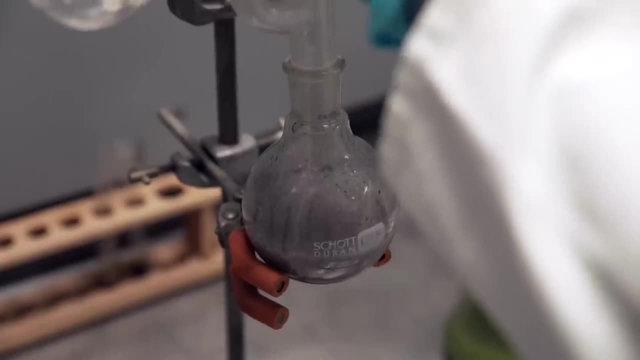 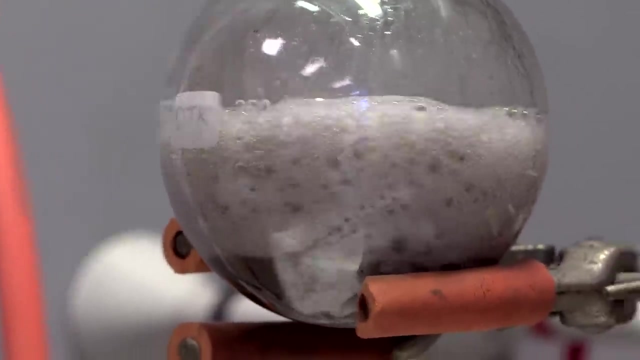 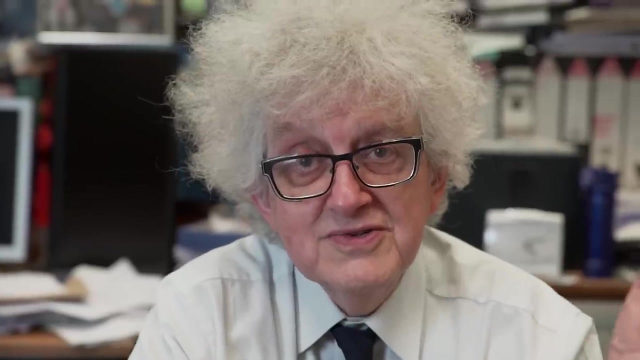 is very volatile. It's a gas. As the hydrogen streams off the reaction, it takes the arsine with it. You're then meant to light the stream of hydrogen coming out of the nozzle at the top of the apparatus. If it's just hydrogen coming out. 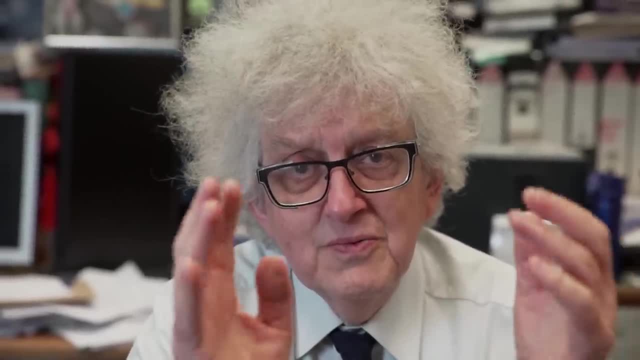 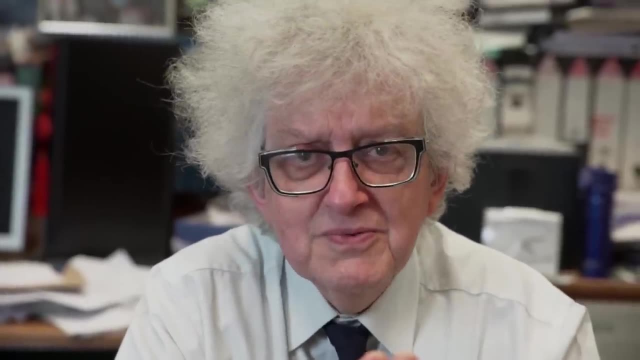 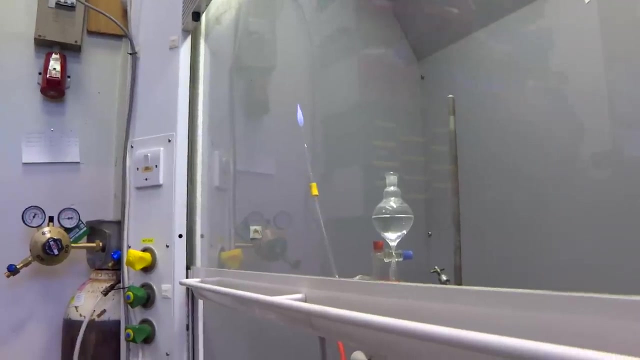 it would be colorless, And Brady was absolutely convinced that we would see a colorless flame and he could tell us how bad we'd been at the experiment. Oh my goodness, It works. I can't believe it worked. That's amazing. 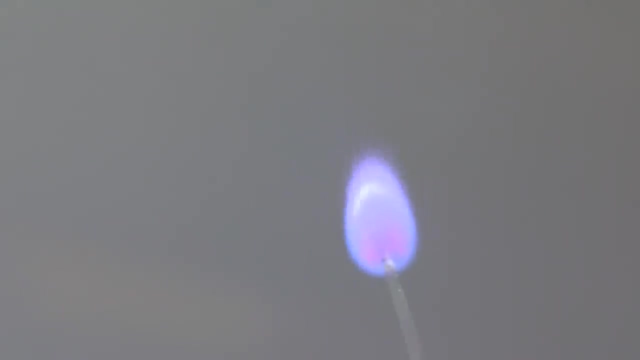 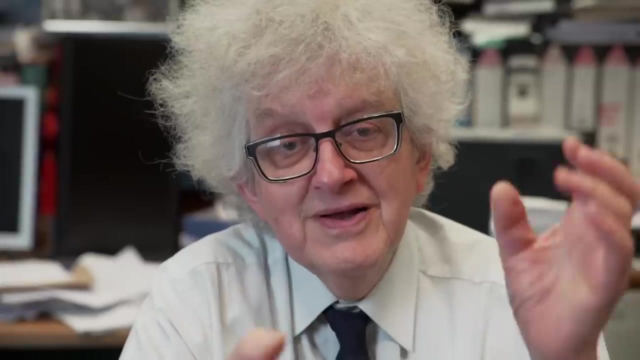 Yes, You happy. Yes, So the murderer is guilty, Martin. Much to all our surprise, the flame came out a beautiful lavender color. Lavender is the color that arsenic burns with. But the real elegance of Marsh's test is that if you put a cold surface, 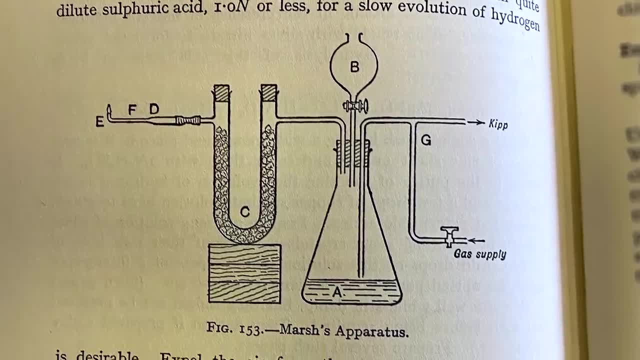 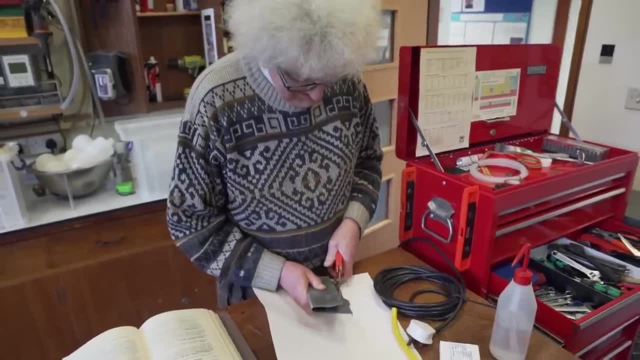 And Neil decided he would like to do Marsh's Test too. The first thing you have to do is to add metallic zinc. I was really excited I was allowed to chop up the zinc. You put in the pieces of zinc into a round bottom flask. 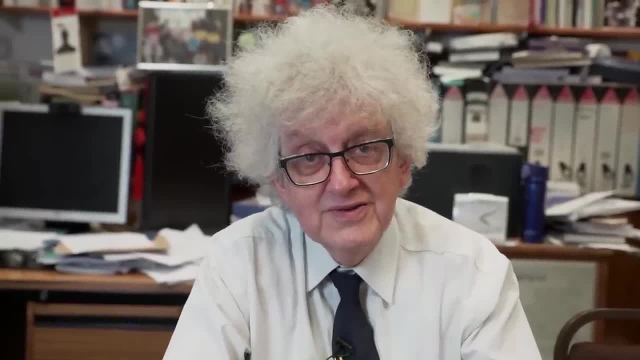 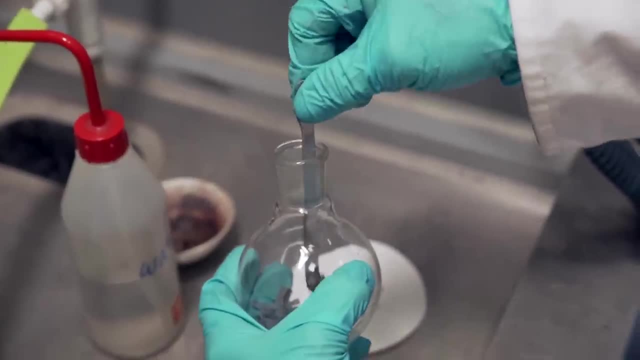 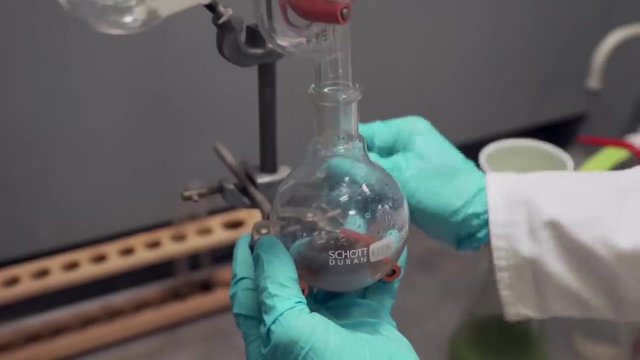 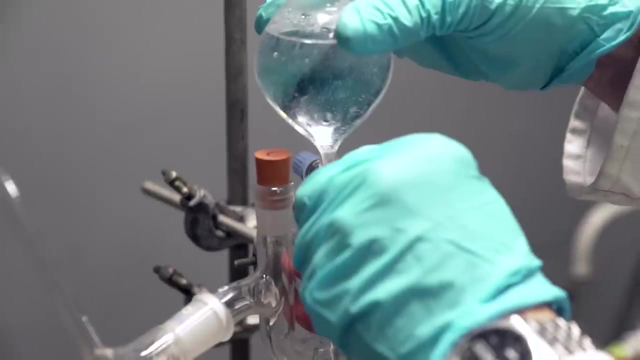 and then you add whatever you think contains arsenic, In our case a small amount of Neil's brown sludge. And then from a dropping funnel you drop in dilute sulfuric acid, and the sulfuric acid reacts with the zinc. 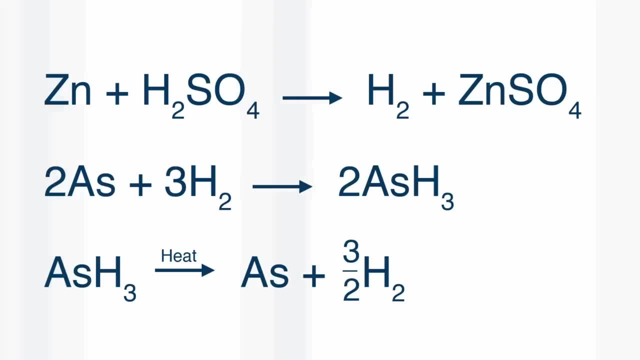 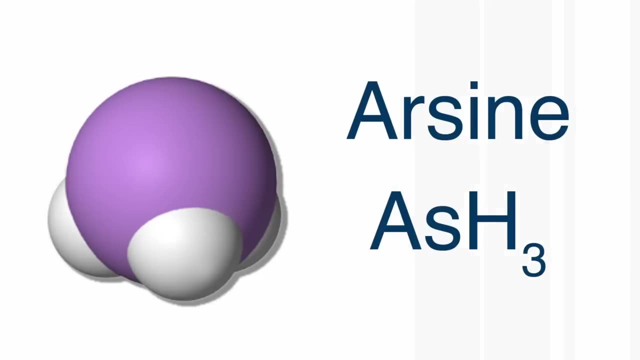 and generates hydrogen. And the hydrogen reacts with the arsenic and makes a compound which has a similar formula to ammonia, but it has three hydrogens attached to arsenic rather than three hydrogens attached to nitrogen which you have in ammonia. And this compound called arsine is very volatile. 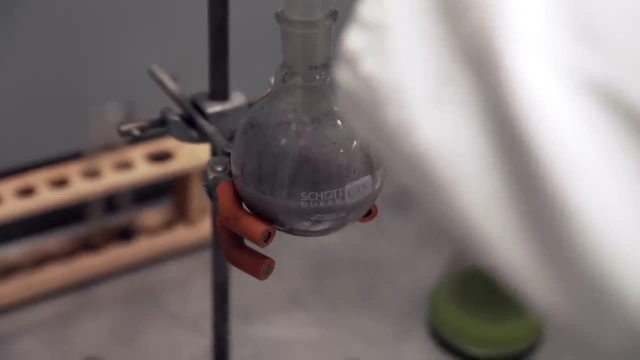 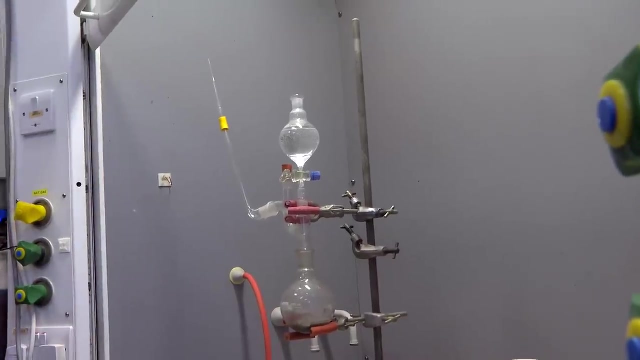 It's a gas, It's invigorous. It's invigorous As the hydrogen streams off the reaction. it takes the arsine with it. You're then meant to light the stream of hydrogen coming out of the nozzle at the top of the apparatus. 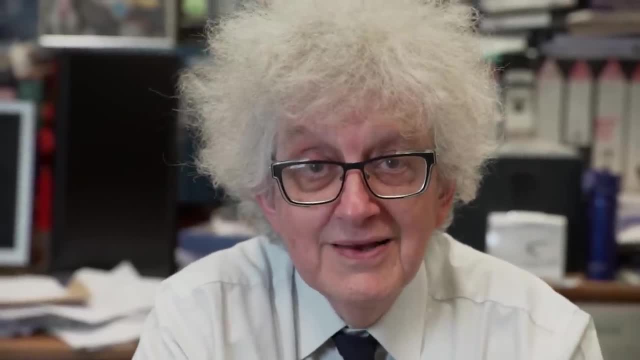 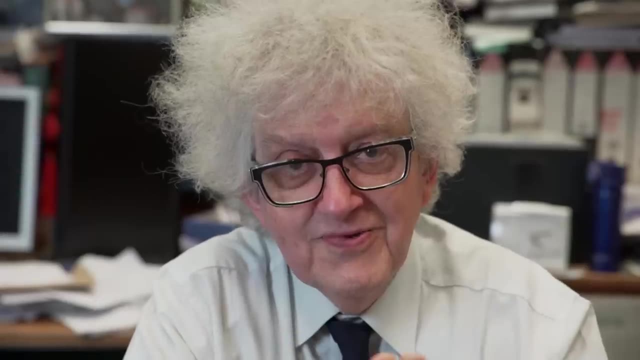 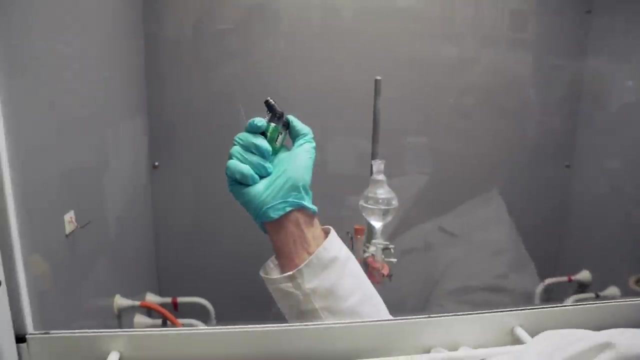 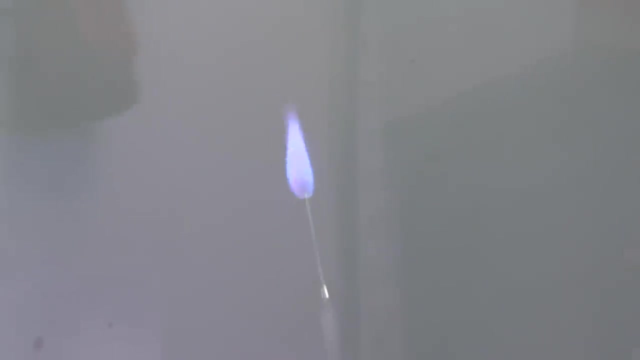 If it's just hydrogen coming out, it would be colorless, And Brady was absolutely convinced that we would see a colorless flame and he could tell us how bad we'd been at the experiment. Oh my goodness, It works. I can't believe it worked. 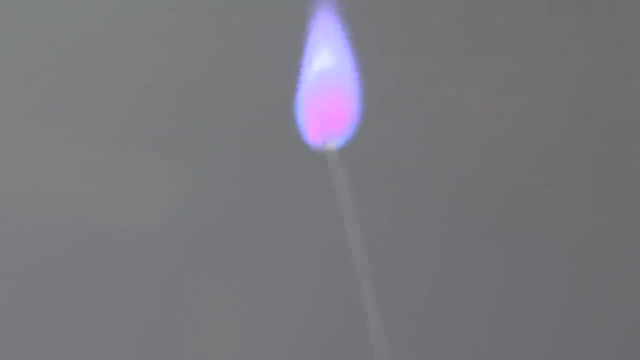 That's amazing. Yes, You happy. Yes, So the murderer is guilty, Martin. Much to all our surprise, the flame came out, a beautiful lavender color. Lavender is the color that arsenic burns with. But the real elegance of Marsh's test is that. 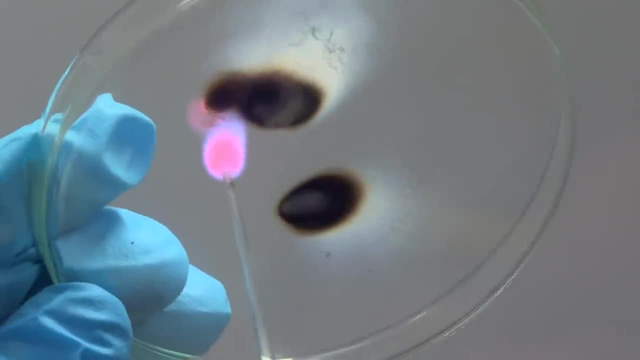 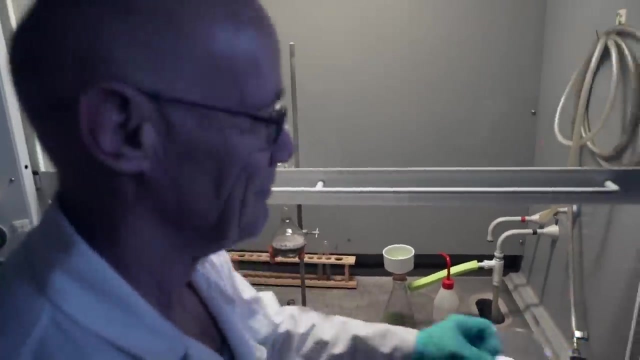 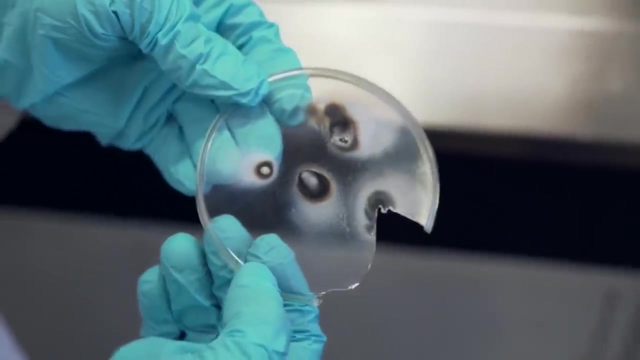 if you put a cold surface, a piece of glass or a piece of porcelain, into the flame, Is that alright? At least we got it on film. The arsine does not burn completely, so you get a thin film of arsenic on the surface. 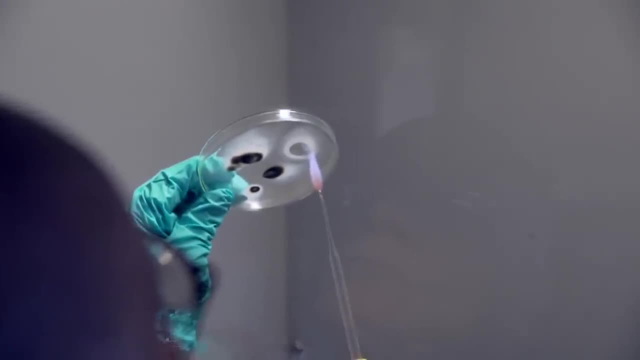 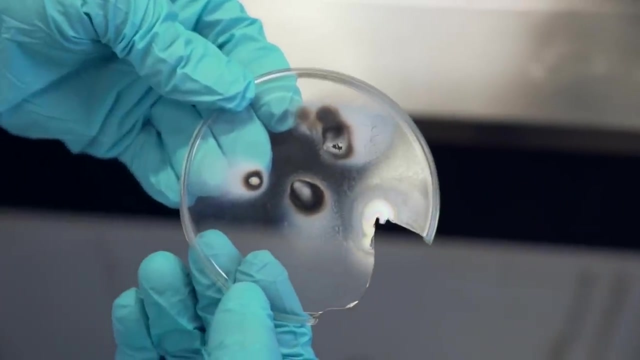 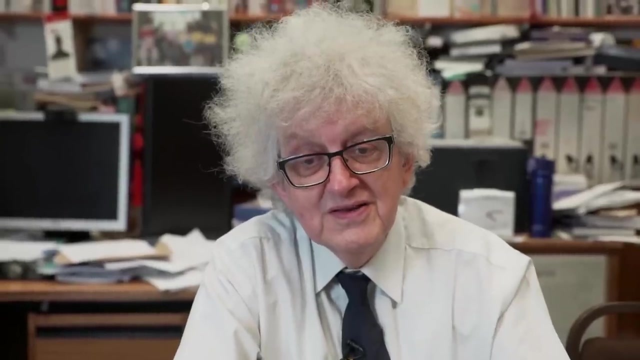 a piece of glass or a piece of porcelain into the flame. Is that all right? At least we got it on film. The arsine does not burn completely, so you get a thin film of arsenic on the surface. The importance of this was that, once the film's there, 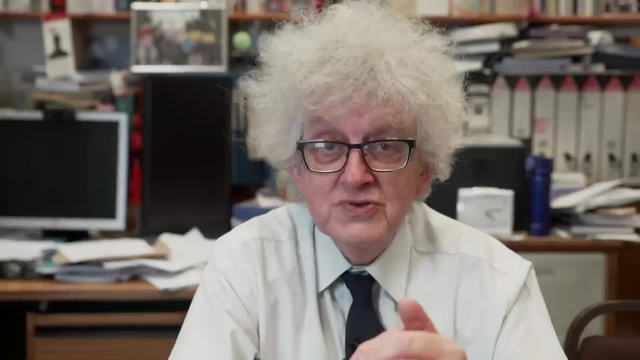 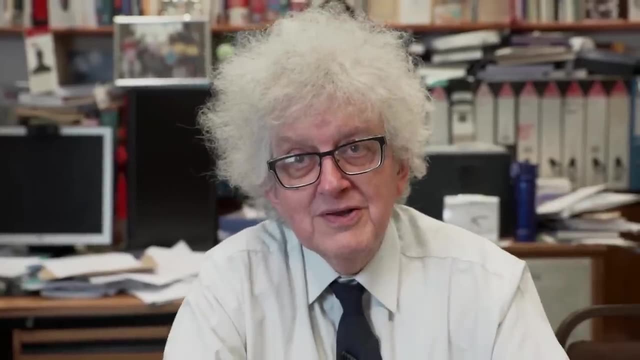 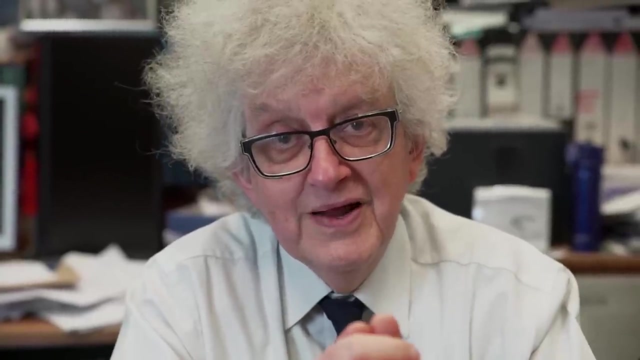 it will stay there so it could be taken to court to be shown as a piece of evidence And you could say: look, arsenic came out of the woman's stomach, or whatever the sample was that you had. There's another, completely different way. 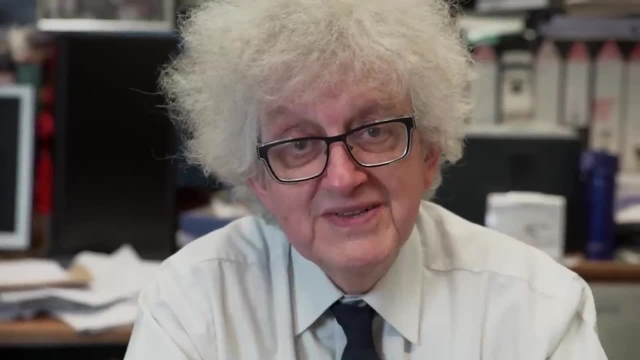 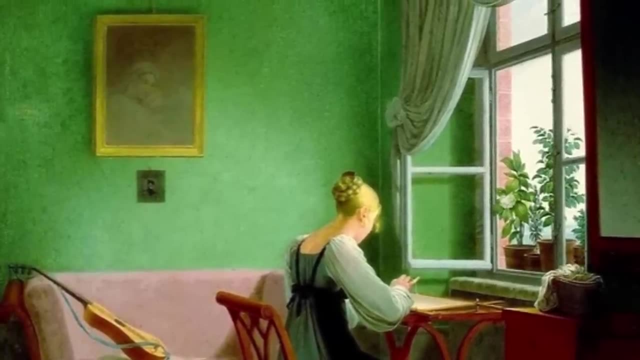 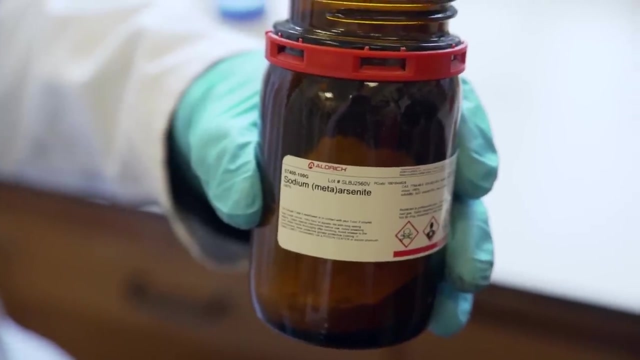 that people in the 19th century were poisoned by arsenic And that was from the green coloring, the green pigment that was used in their wallpaper. This green pigment is a copper salt called Schiele's Green. It is made by taking a solution. 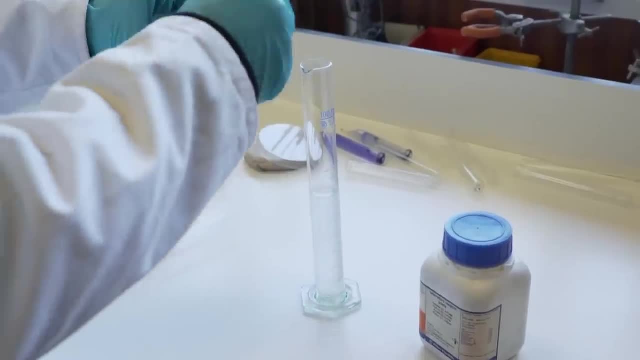 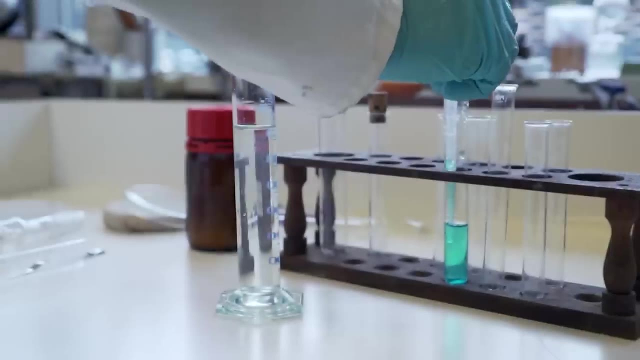 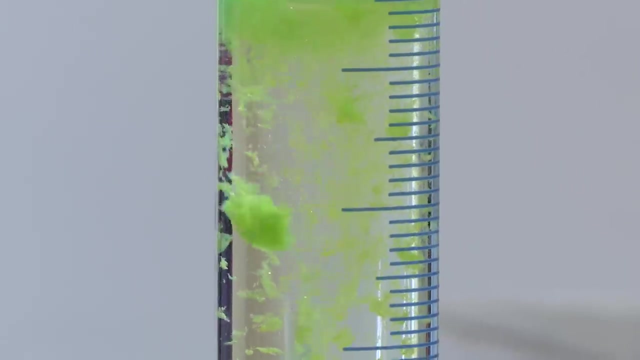 of sodium metarsenite, which is colorless, and dropping in copper sulfate, which is blue. I've done this reaction several times, but I haven't done it for a long time And I was really surprised quite how beautiful it is. 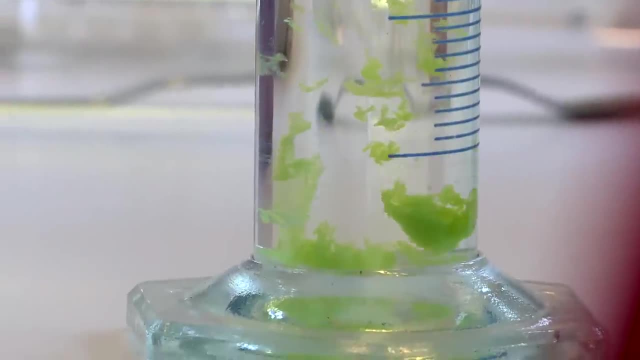 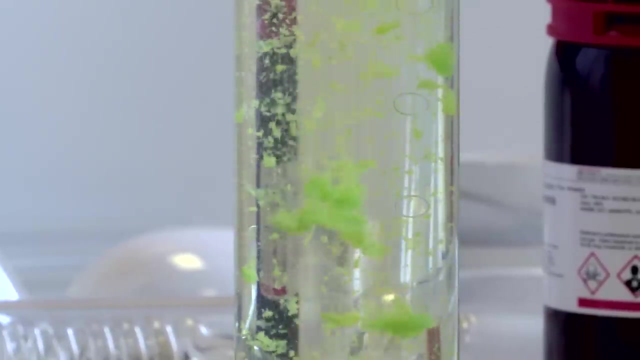 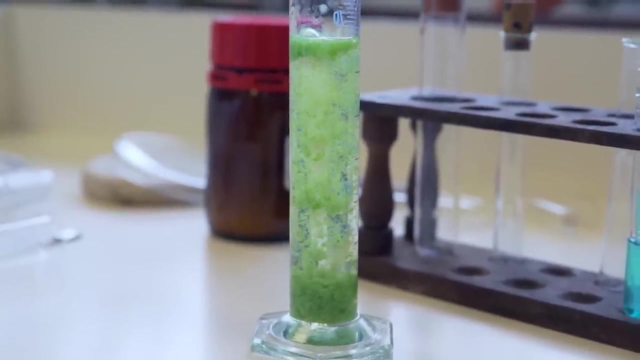 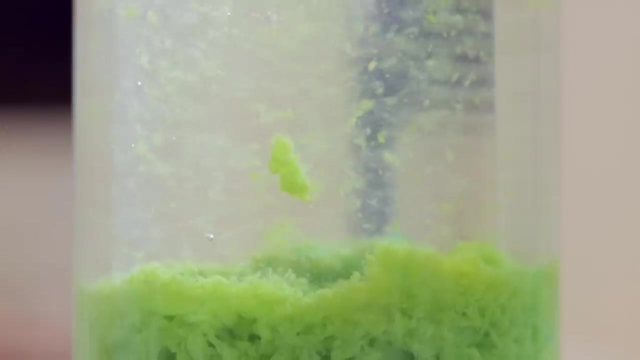 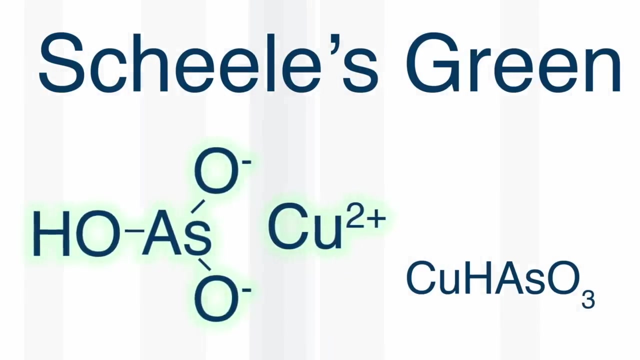 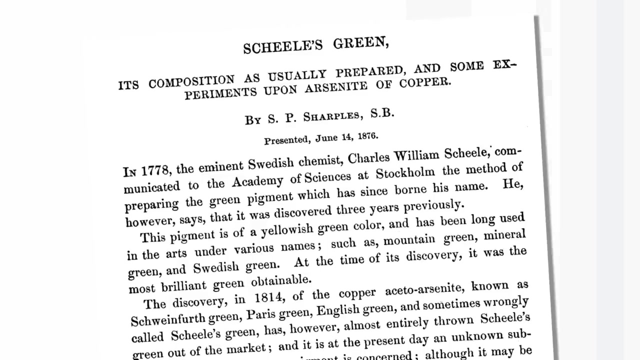 seeing this green solid forming. Schiele's Green was used quite widely. This would have been fine, except in those days people were really frightened of drafts And they used to close all the windows and doors and have very stuffy rooms which were not very well heated. 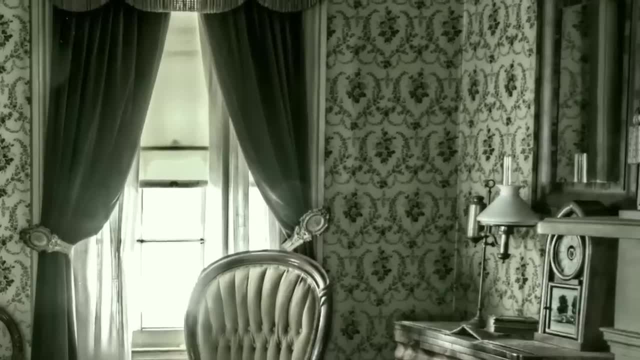 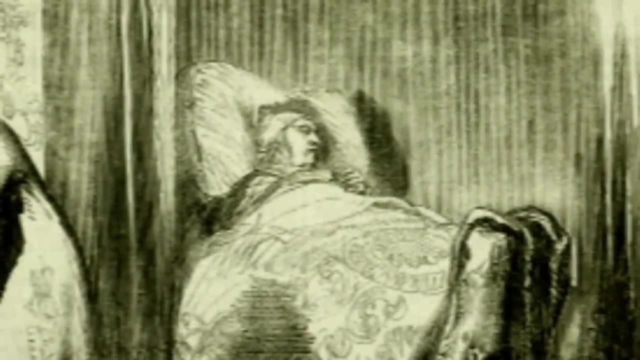 So, particularly at night when they were asleep, there was a lot of condensation and mold would grow on the wallpaper, And so the mold growing on your wallpaper could create a gas containing arsenic, which, if you were lying asleep in this airless room, 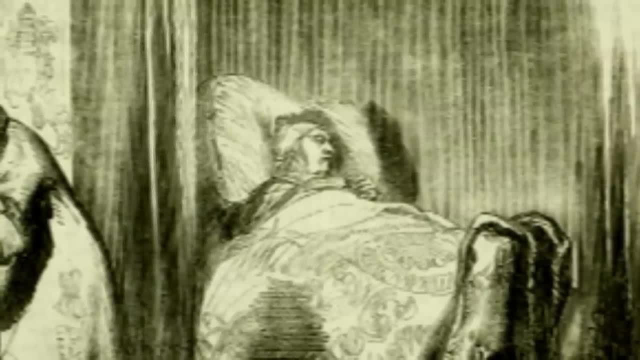 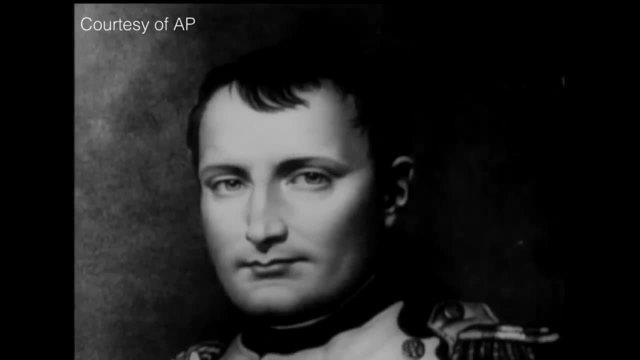 over a period of just one night would be enough to kill you. In October 1815,, Napoleon Bonaparte was brought a prisoner to the island of St Helena in the South Atlantic. Here he was to spend the last six years of his life. 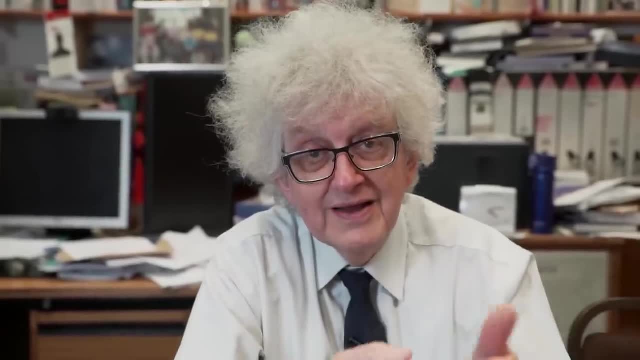 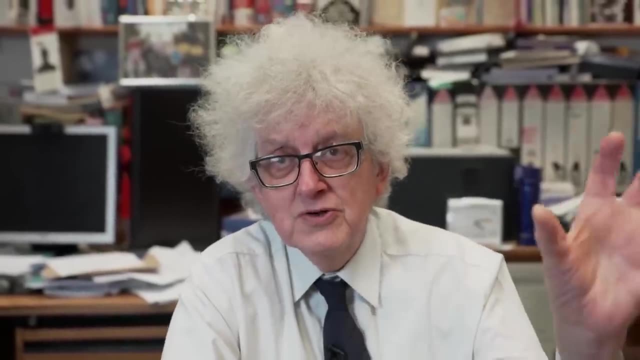 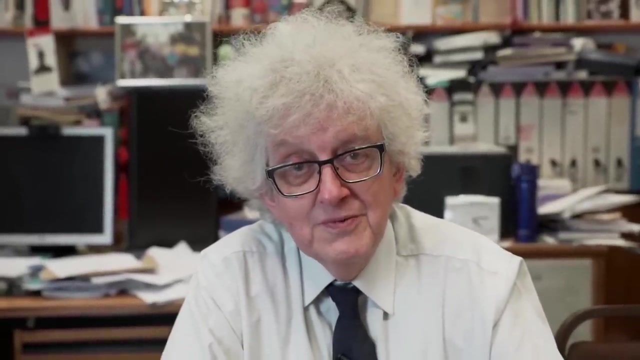 The importance of this was that once the film's there, it will stay there, so it could be taken to court to be shown as a piece of evidence And you could say: look, arsenic came out of there, came out of the woman's stomach, or whatever the sample was that you had. 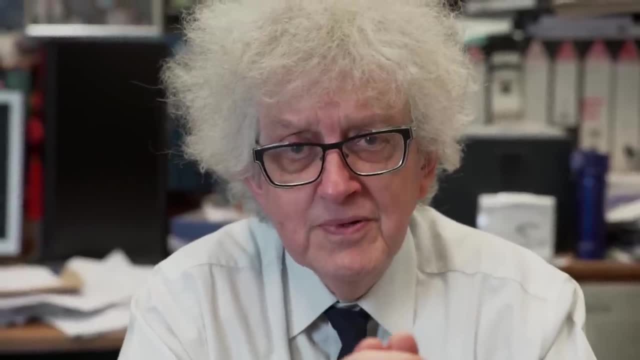 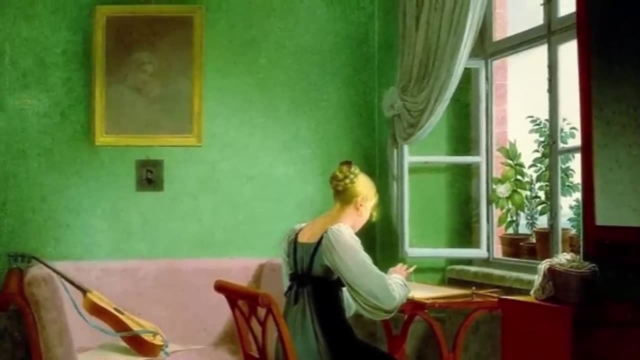 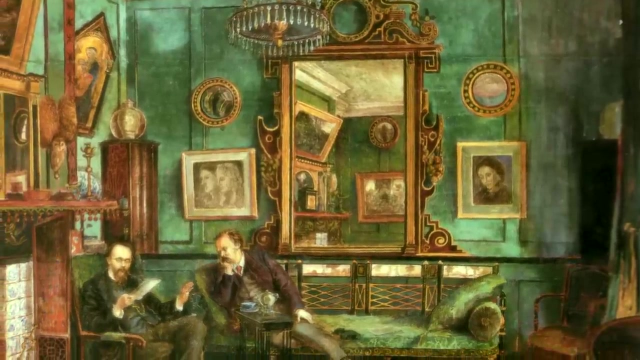 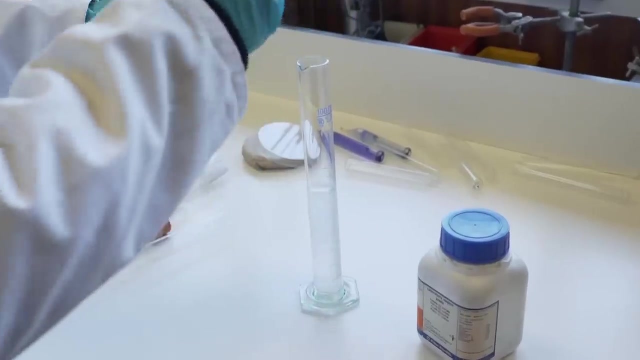 There's another, completely different way that people in the 19th century were poisoned by arsenic, and that was from the green coloring, the green pigment that was used in their wallpaper. This green pigment is a copper salt called Schiele's Green. It is made by taking a solution of sodium meta-arsenite, which is colorless and dropping. 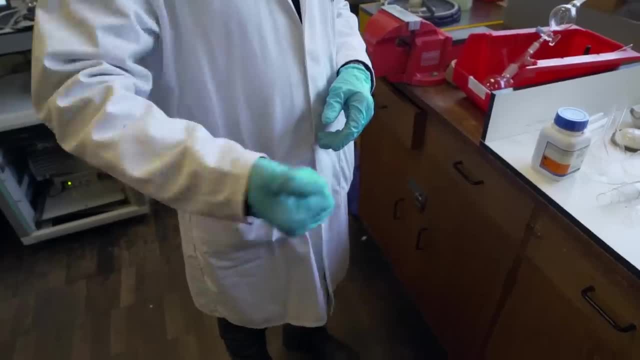 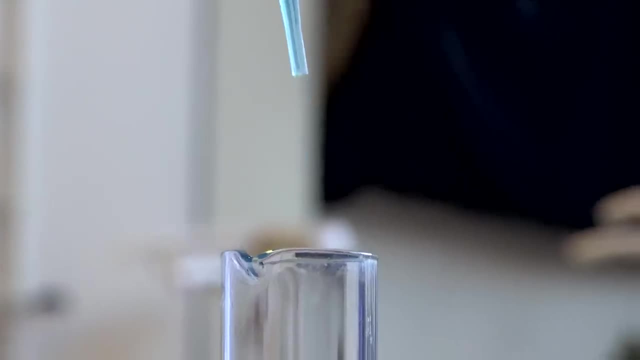 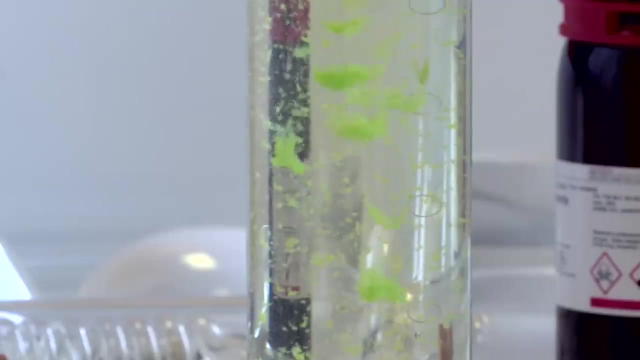 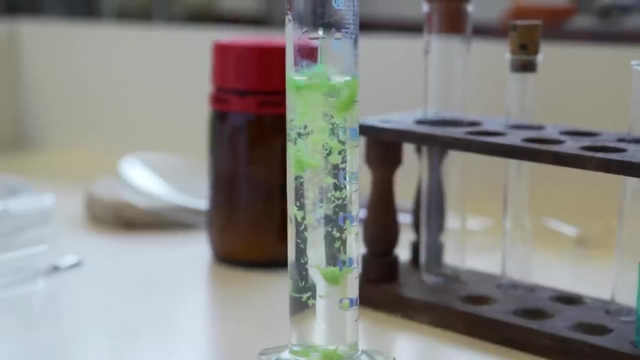 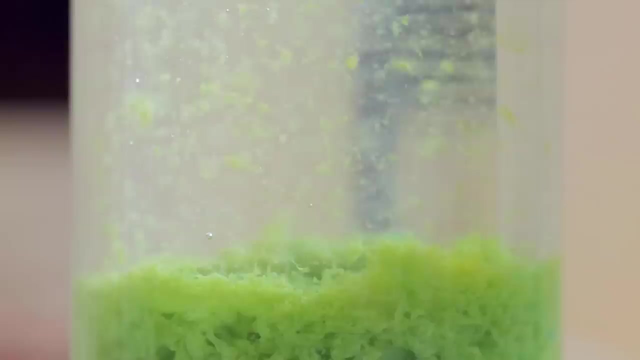 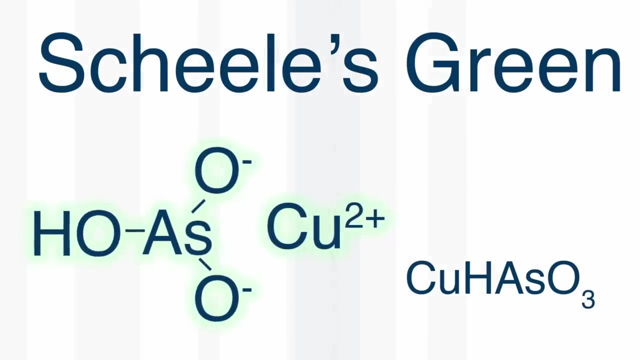 in copper sulfate, which is blue. I've done this reaction several times, but I haven't done it for a long time and I was really surprised quite how beautiful it is seeing this green solid forming. Schiele's Green was used quite widely. This would have been fine, except in those days people were really frightened of draughts. 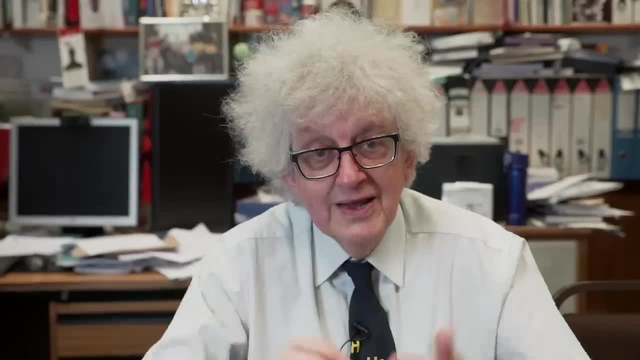 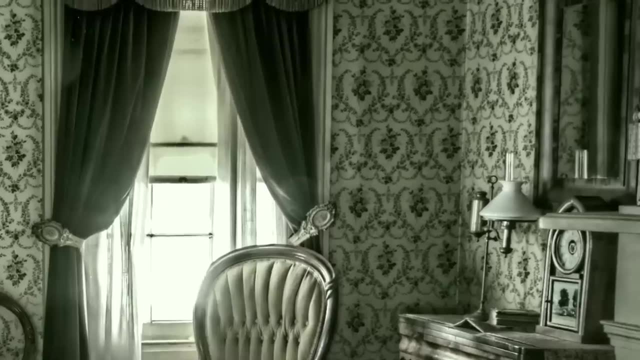 and they used to close all the windows. They would close all the doors and have very stuffy rooms which were not very well heated. So particularly at night when they were asleep, there was a lot of condensation and mold would grow on the wallpaper. 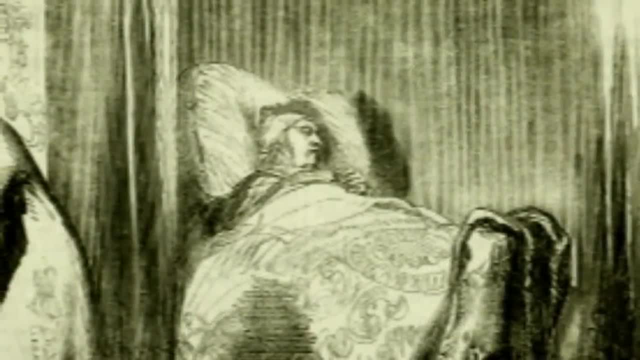 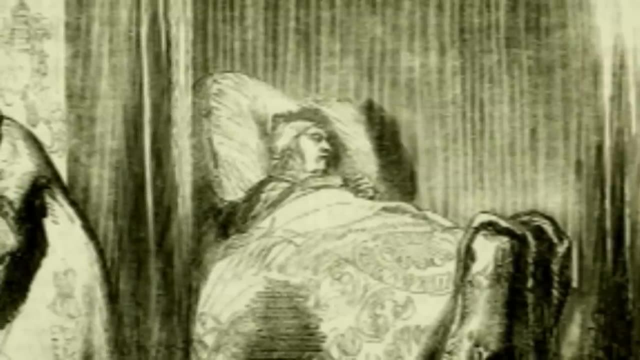 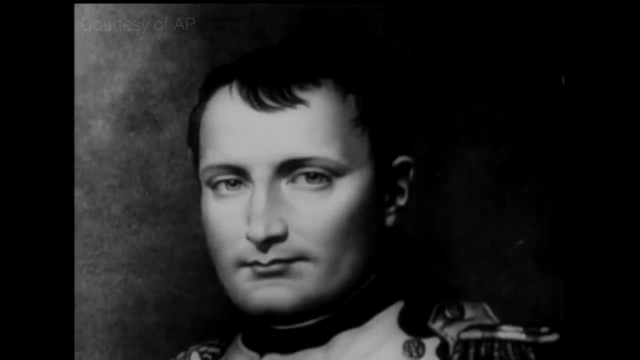 And so the mold growing on your wallpaper could create a gas containing arsenic which, if you were lying asleep in this airless room over a period of just one night, would be enough to kill you. In October 1815, Napoleon Bonaparte was brought a prisoner to the island of St Helena in the 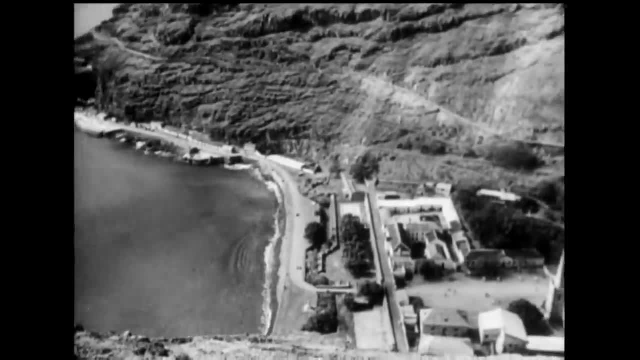 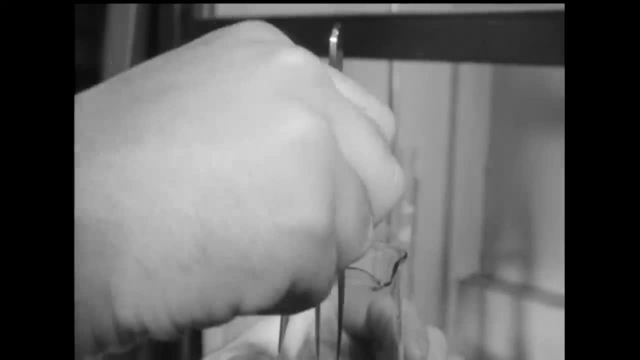 South Atlantic. Here he was to spend the last six years of his life. Here he died on the 5th of May 1821.. Examination was made of specimens of hair said to have been taken from the head of Napoleon both before and after he died. 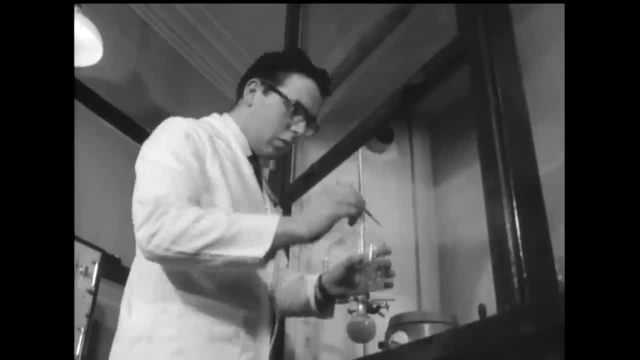 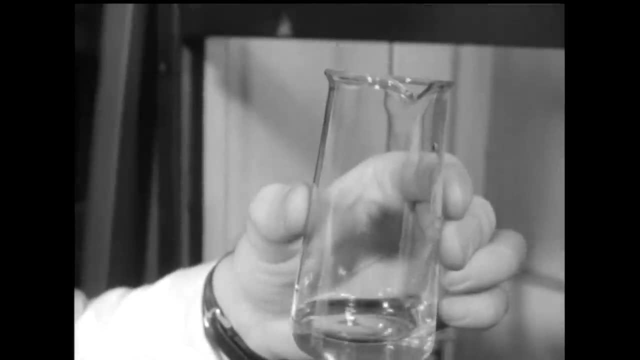 Here he died on the 5th of May 1821.. Examination was made of specimens of hair said to have been taken from the head of Napoleon both before and after he died. The results established the presence of arsenic. My friend David Jones. 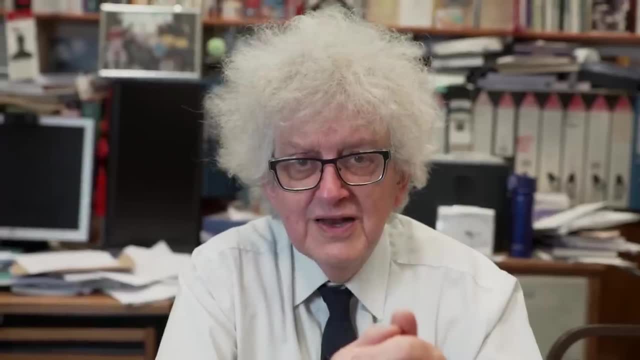 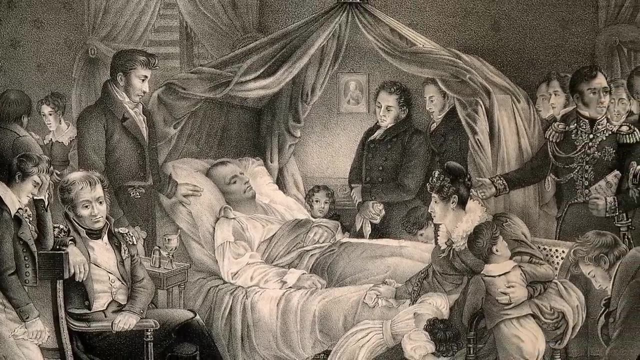 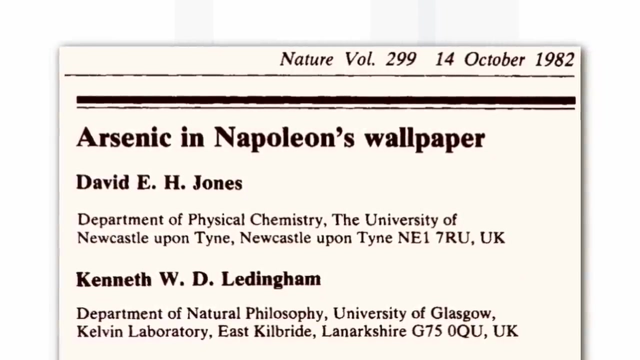 who was an expert in really weird chemical facts, wondered whether the stories of Napoleon being poisoned with arsenic by the wicked British could in fact be due to mold on the wallpaper in his house on the island of St Helena where he was exiled. 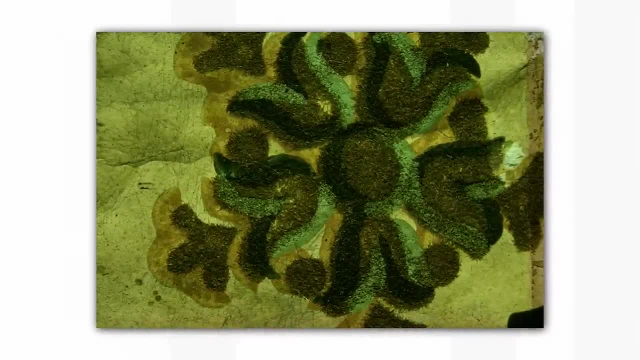 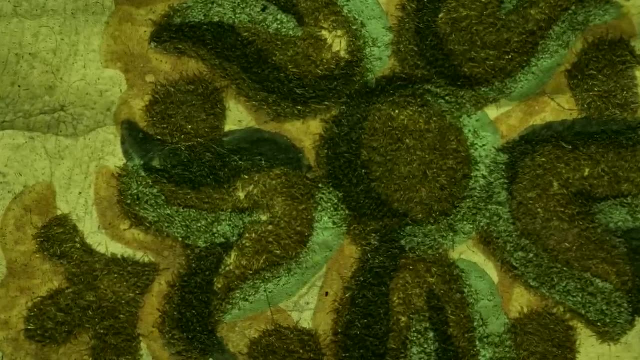 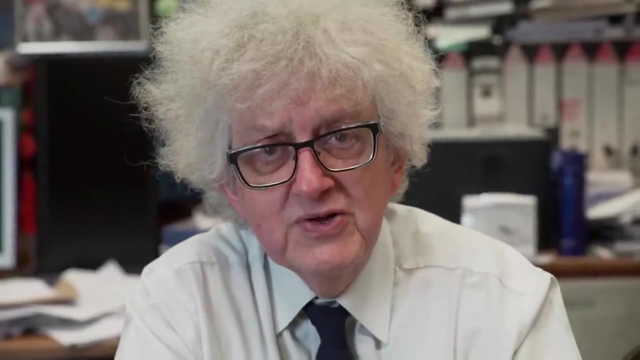 And, remarkably, David managed to get hold of a sample of Napoleon's wallpaper which had some green marks on it And he could analyze this and show that it did indeed contain arsenic. And there was enough arsenic in Napoleon's wallpaper to explain the arsenic. 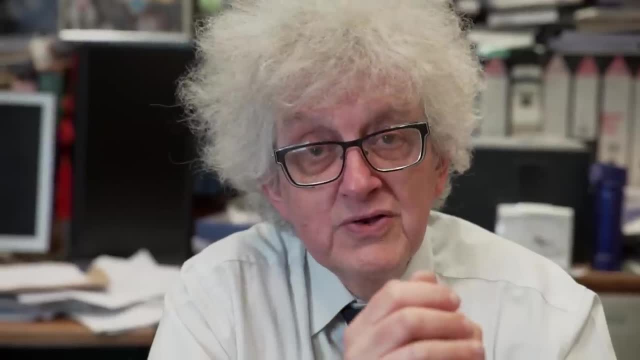 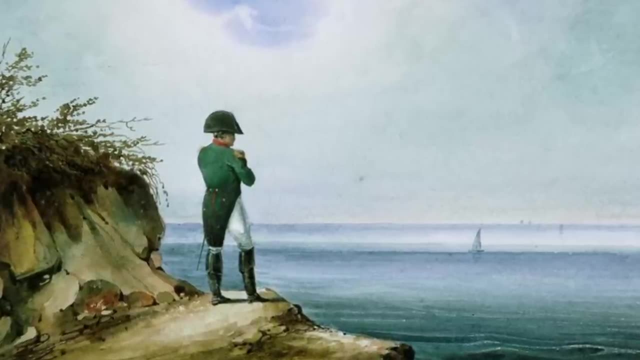 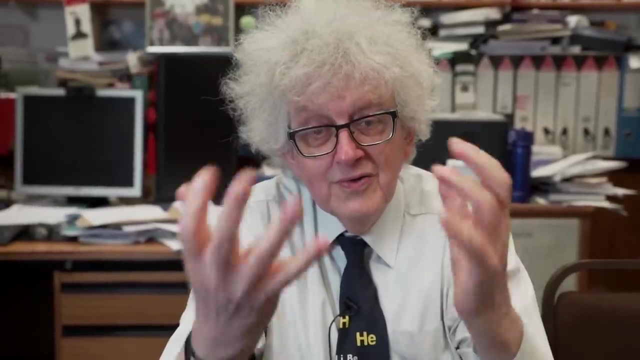 that had been found in his hair, but not enough to have killed him. So, according to David's experiments, the British did not poison Napoleon, but he just felt unwell because of his green wallpaper. The action of mold on arsenic compound. 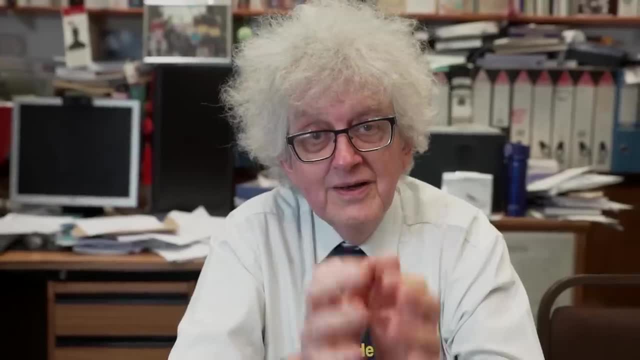 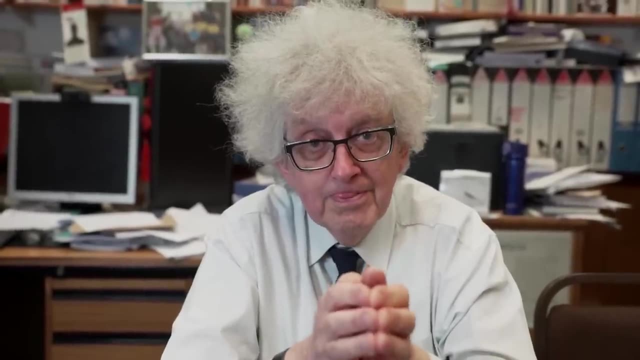 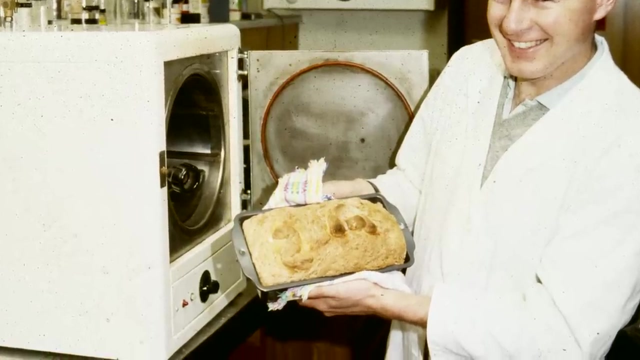 was exploited for real chemistry by an Australian chemist called Bruce Wilde and his technician Paul Guggen. They did a really unique experiment. They got some bread and injected it with an arsenic compound that was not volatile and then put the bread in a large container. 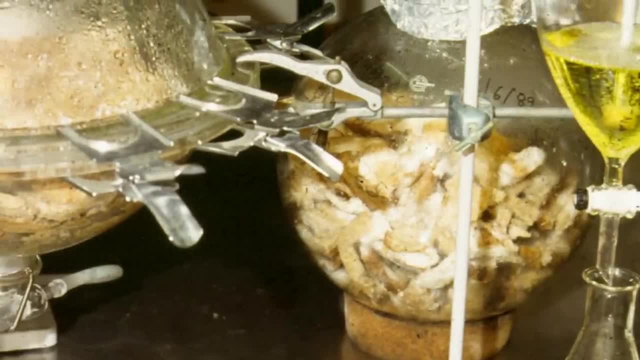 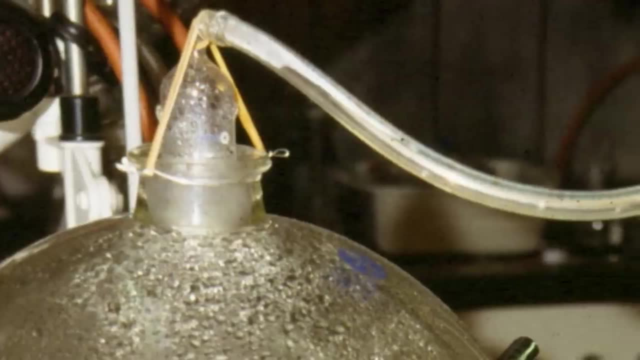 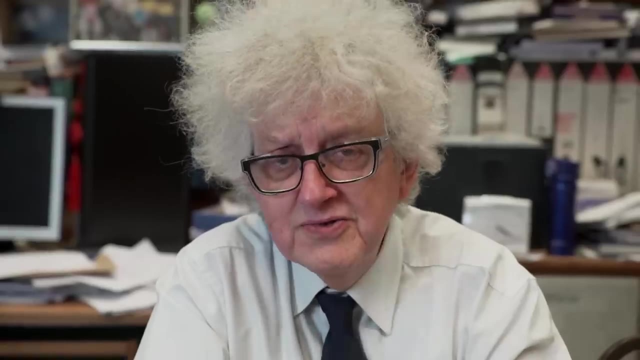 and let mold grow on it. The mold converted the arsenic compound into a volatile compound, a gas. Then they led this through a tube into a solution and they got a yellow solution of a new complex. And the reason they used the mold is because, unlike human chemists, 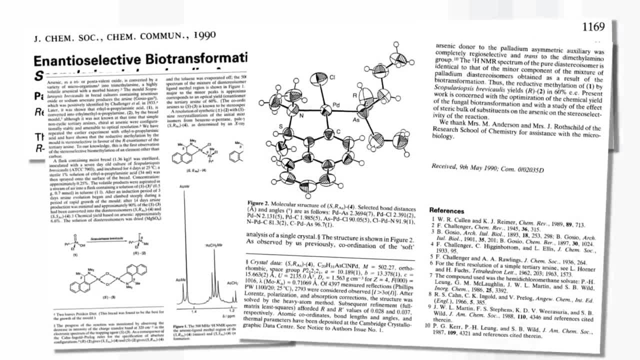 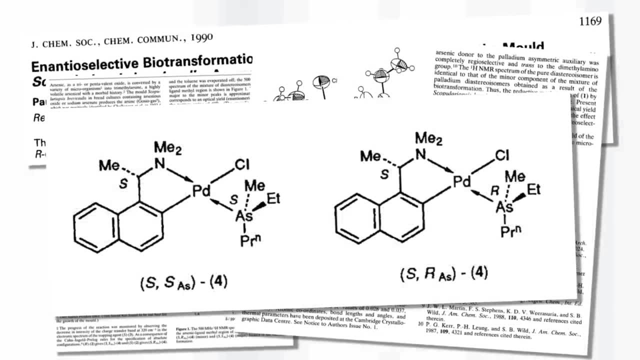 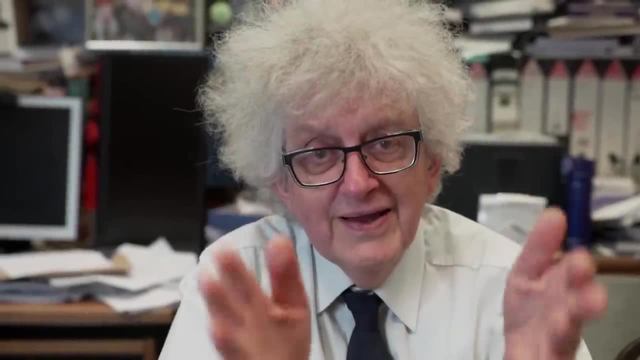 the mold could produce a so-called optically active compound, that is, a left-handed version of the molecule without the right-handed one, whereas ordinary chemists produce both at the same time. And they published a great paper and they had an extraordinary photo of Paul the technician. 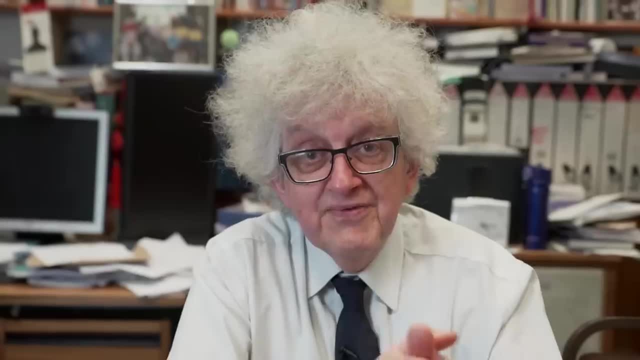 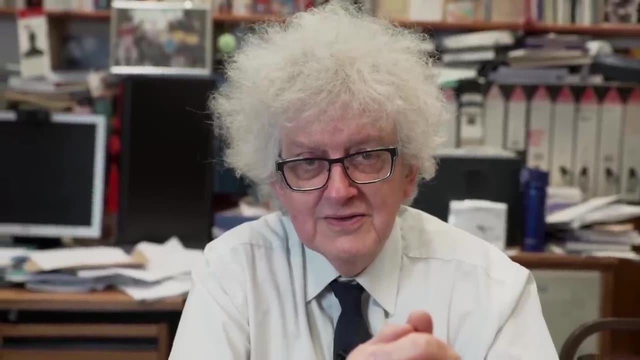 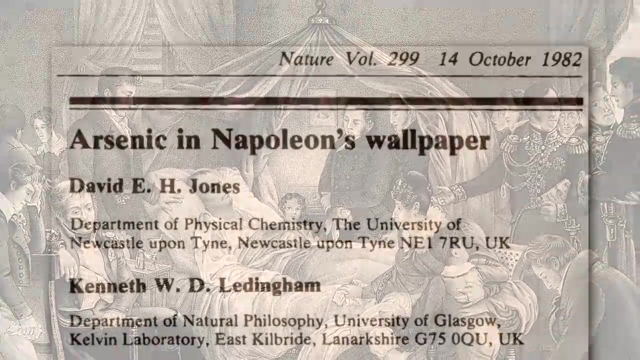 The results established the presence of arsenic. My friend David Jones, who was an expert in really weird chemical facts, Wondered whether the stories of Napoleon being poisoned with arsenic by the wicked British could in fact be due to mold on the wallpaper in his house on the island of St Helena, where 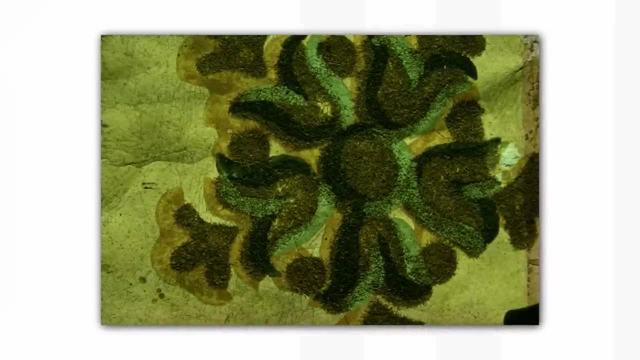 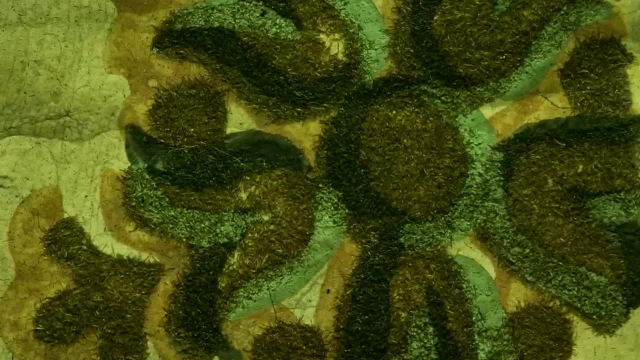 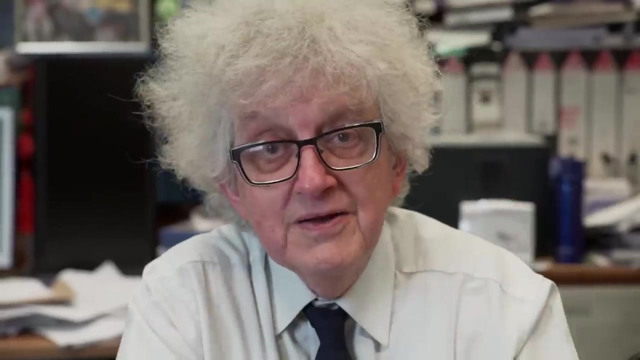 he was exiled. Remarkably, David managed to get hold of a sample of Napoleon's wallpaper which had some green marks on it, And he could analyze this and show that it did indeed contain arsenic. And there was enough arsenic in Napoleon's wallpaper to explain the arsenic that had. 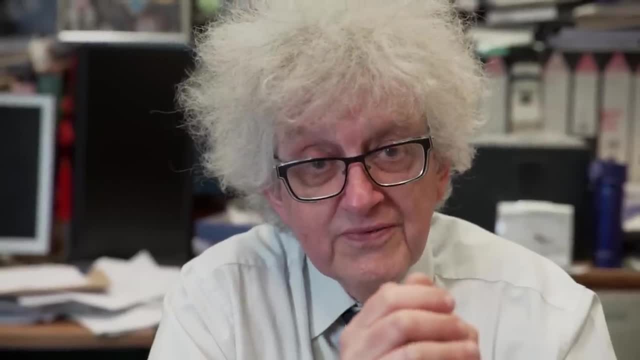 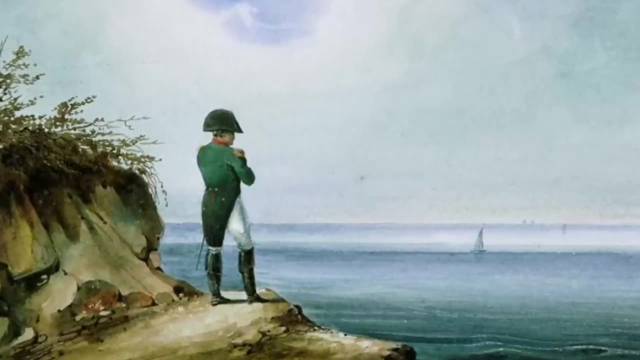 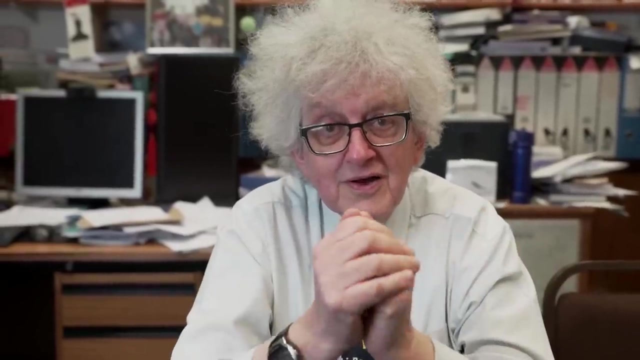 been found in his hair, But not enough to have killed him. So, according to David's experiments, the British did not poison Napoleon, but he just felt unwell because of his green wallpaper. The action of mold on arsenic compound was exploited for real chemistry by an australian. 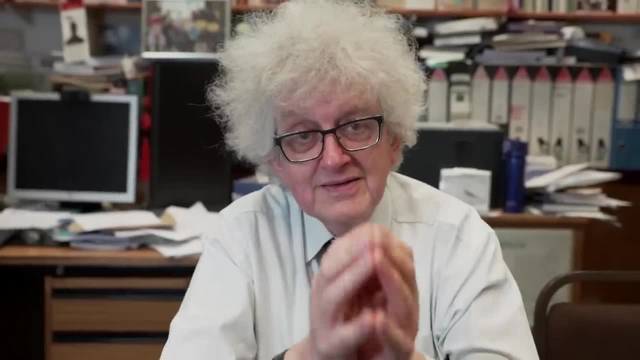 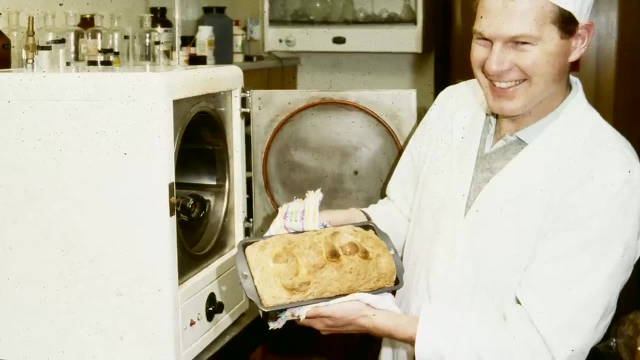 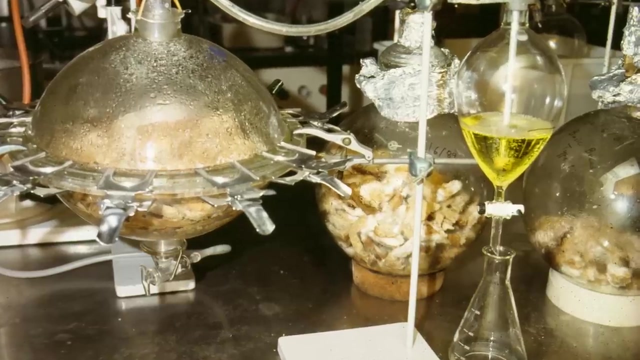 chemist called Bruce Wilde and his technician, Paul Guggen. They did a really unique experiment. They got some bread and injected it with an arsenic compound that was not volatile, And then put the bread in a large container and let mold grow on it. 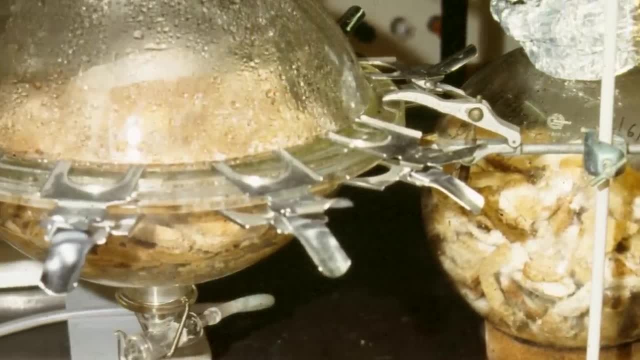 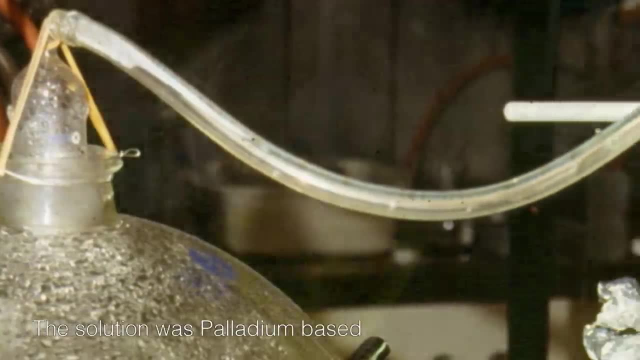 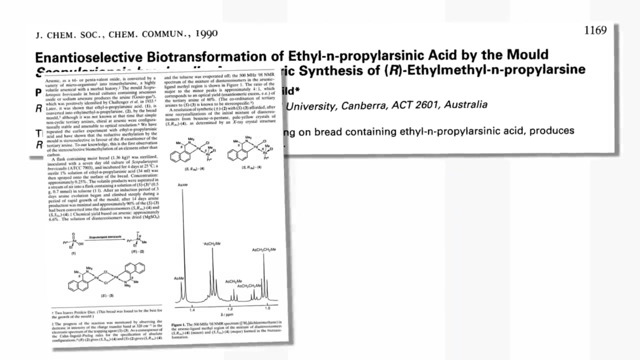 The mold converted the arsenic compound into a volatile compound, a gas. Then they led this through a tube Into a solution And they got a yellow solution of a new complex. And the reason they used the mold is because, unlike human chemists, the mold could produce. 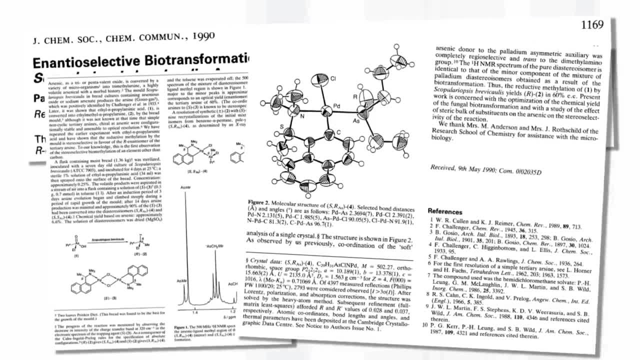 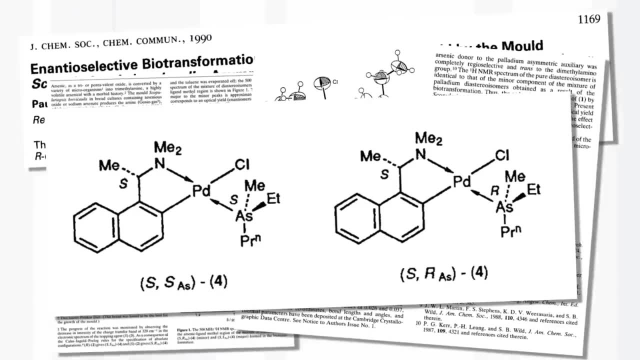 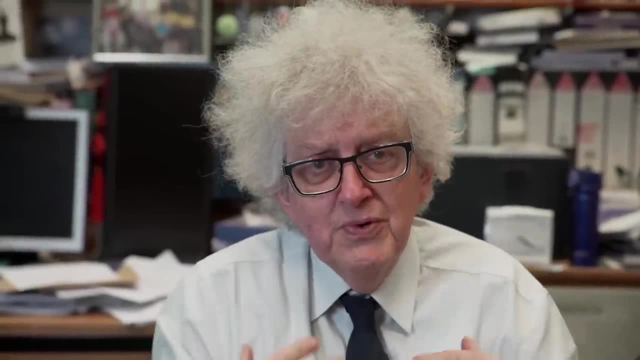 a so-called optically active compound, that is, a left-handed version of the molecule without the right-handed one, Whereas ordinary chemists produce both at the same time. And they published a great paper And they had an extraordinary photo of it, A photo of Paul the technician holding this loaf of bread full of arsenic. 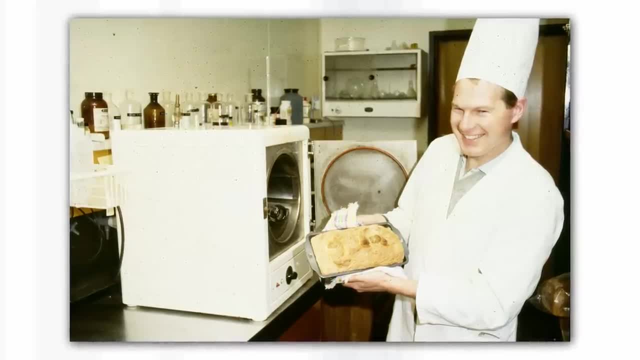 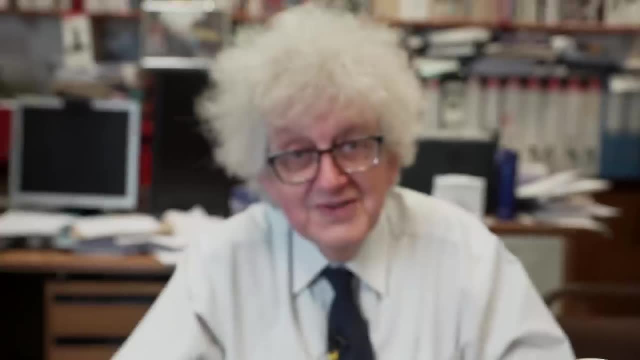 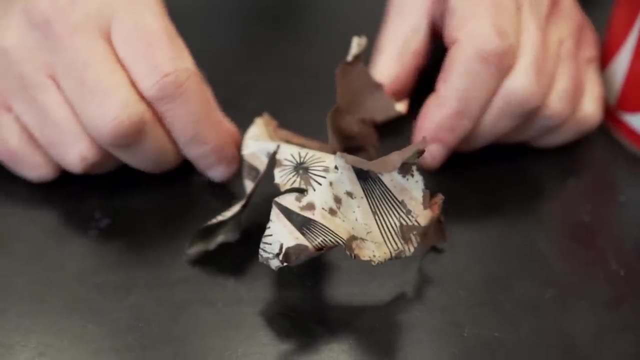 holding this loaf of bread full of arsenic. I dread to think what their safety assessment looked like. This piece of metal has an extraordinary story about it which involves arsenic. When I first came here to Nottingham, one of my colleagues, Mike 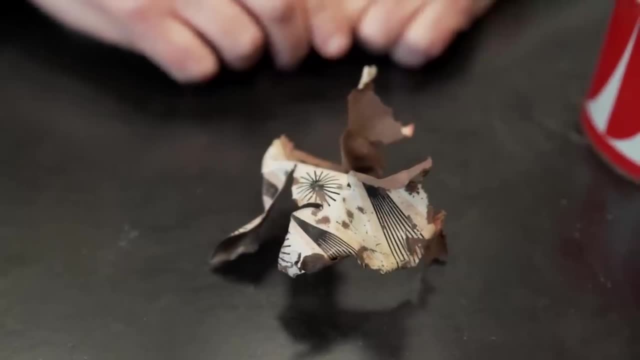 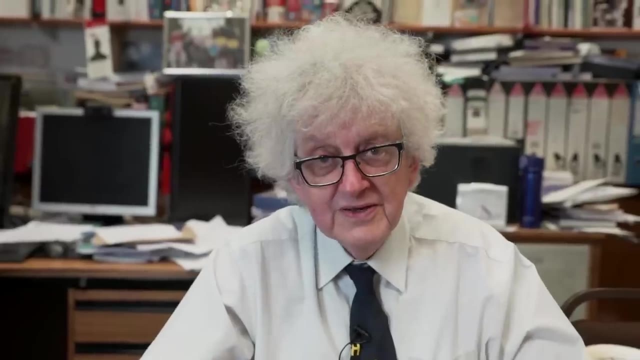 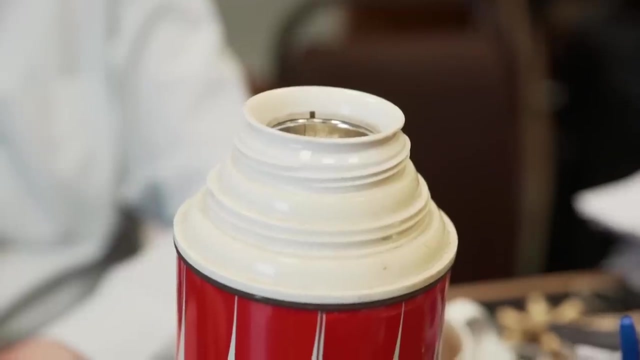 was studying the reactions of arsenic with liquid fluorine. If it's done carefully, this is a nice controlled reaction. You have to do it with the apparatus cooled in liquid nitrogen, So he was doing the reaction inside a thermos flask that looks like this. 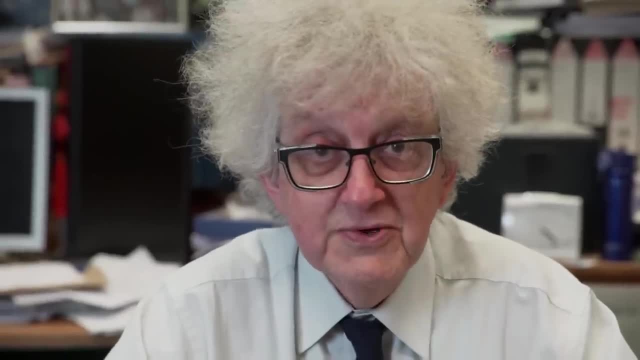 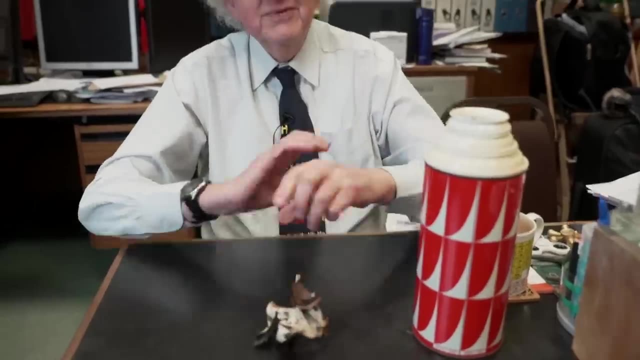 And something went wrong and there was an enormous explosion. All that was left of the thermos was the plastic top and this piece of metal. Everything else was distributed around the lab, But I think the importance of this is to show you that arsenic 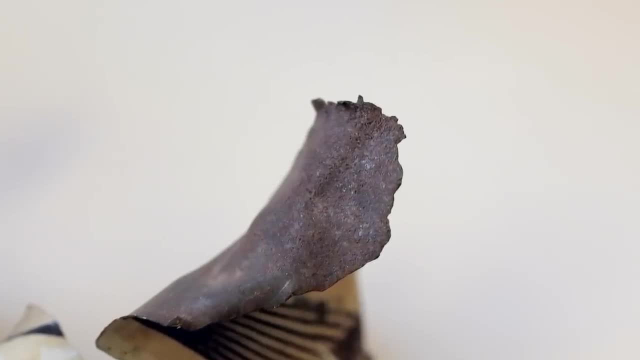 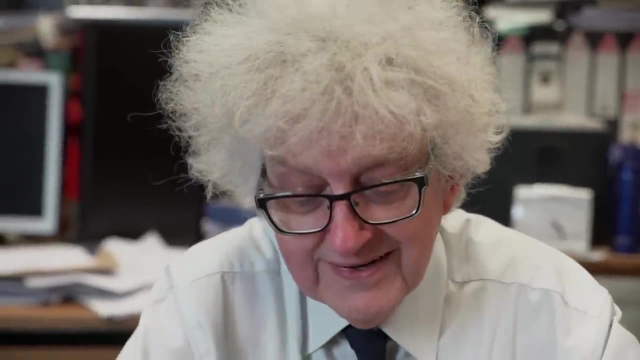 if you get it in the right state- or perhaps I should say in the wrong state- can react very violently. I went into the lab before it had been cleaned up and retrieved this because I was just so amazed by it And I used to use it. 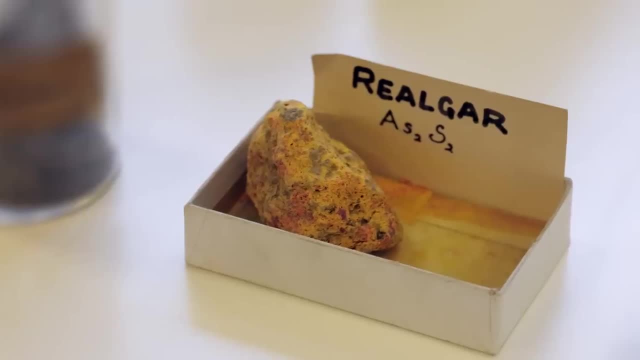 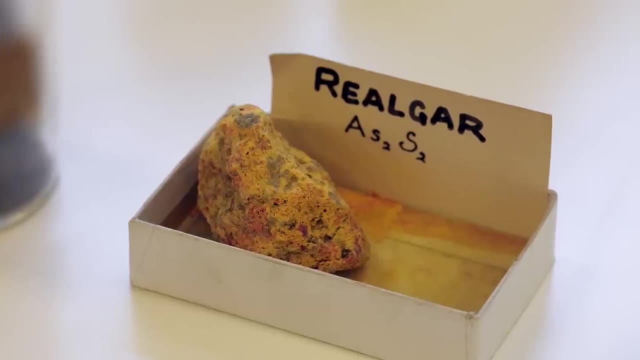 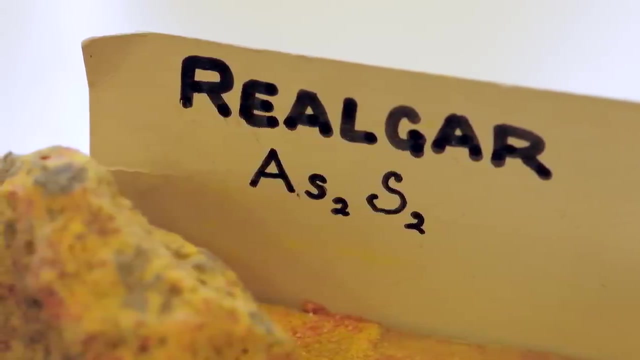 when I was teaching about arsenic chemistry. Apparently, metallic arsenic can occasionally be found in natural minerals, but usually it's found as compounds, And in our store we have a sample of one of the minerals containing arsenic that's called Rialgar. 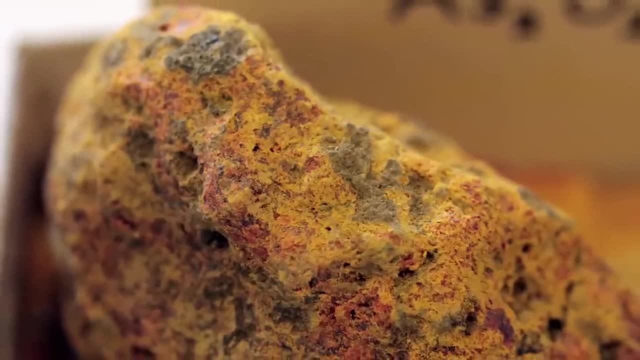 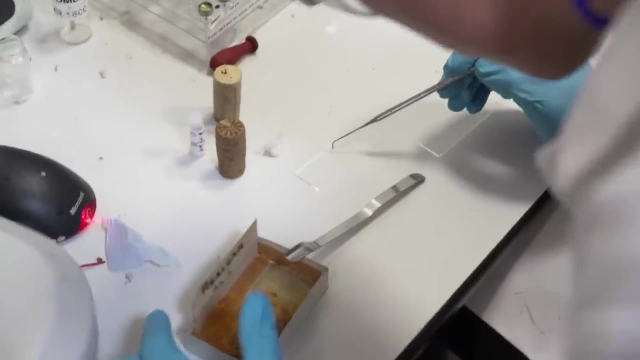 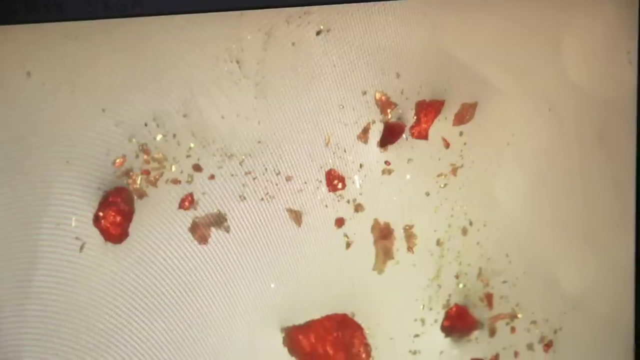 It's an arsenic sulphide which has really very nice red crystals. Unfortunately, our sample has rather small crystals, but if you look at them under a microscope you can see really nice red crystals which are of arsenic sulphide, And this is probably why. 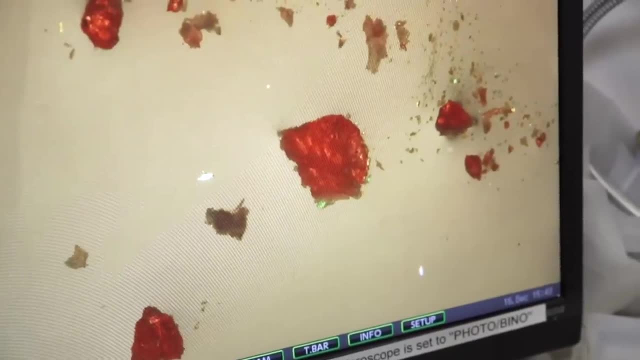 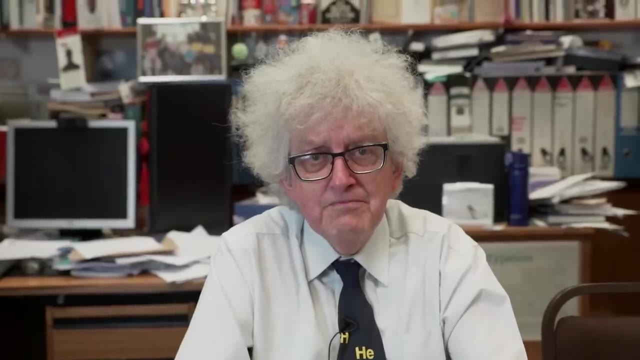 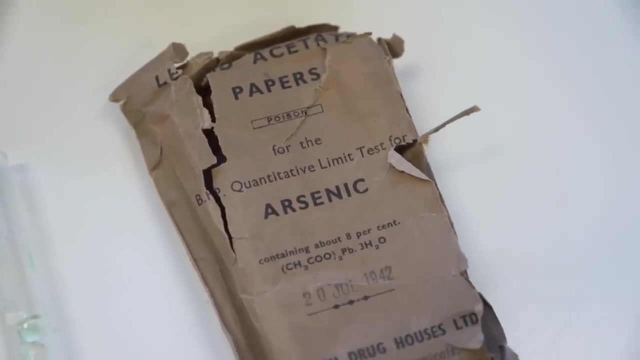 arsenic compounds were known even in ancient times because of these brightly coloured minerals. While we were filming, Neil found some amazing old papers- lead acetate papers- for testing for arsenic. They were labelled 20th July 1942, before any of us were born. 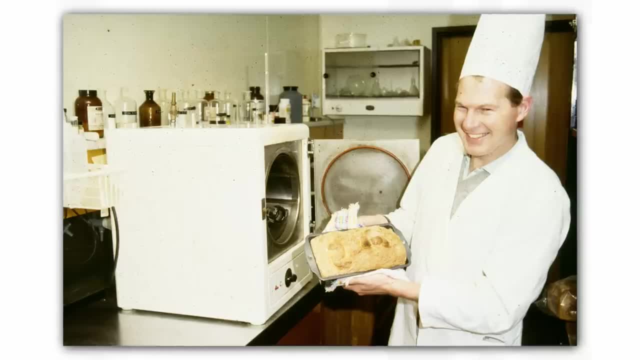 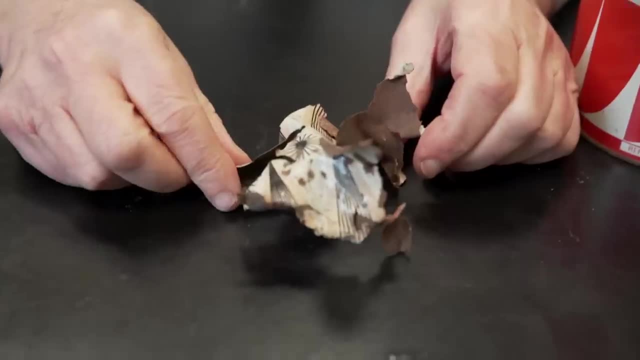 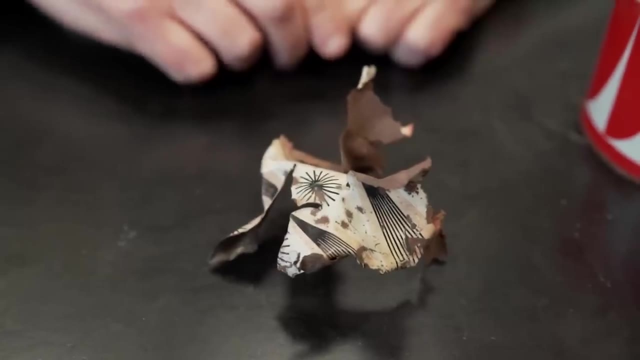 I dread to think what their safety assessment looked like. This piece of metal has an extraordinary story about it, which involves arsenic. When I first came here to Nottingham, one of my colleagues, Mike, was studying the reactions of arsenic with liquid fluorine. 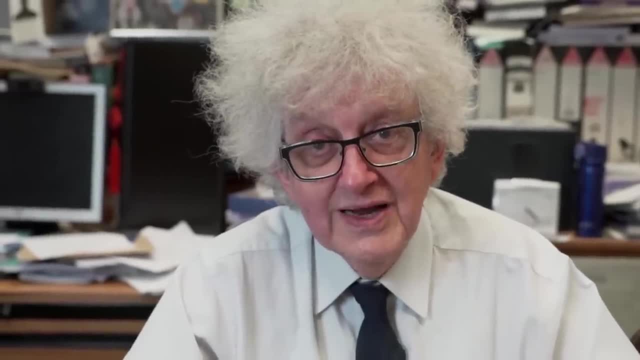 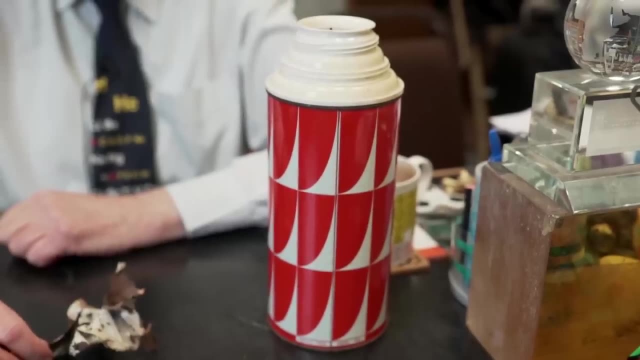 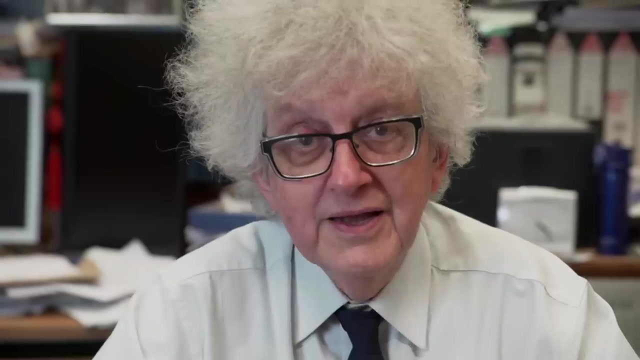 If it's done carefully, this is a nice controlled reaction. You have to do it carefully. You have to do it with the apparatus cooled in liquid nitrogen. So he was doing the reaction inside a thermos flask that looks like this And something went wrong. 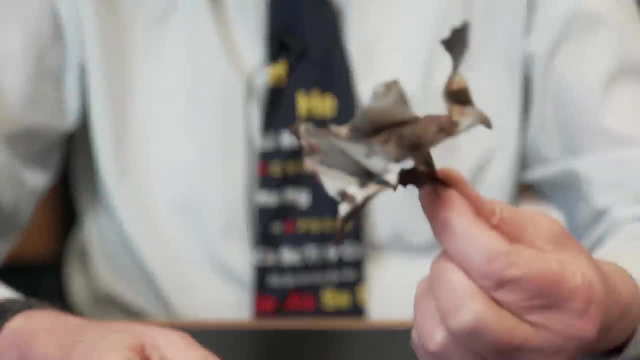 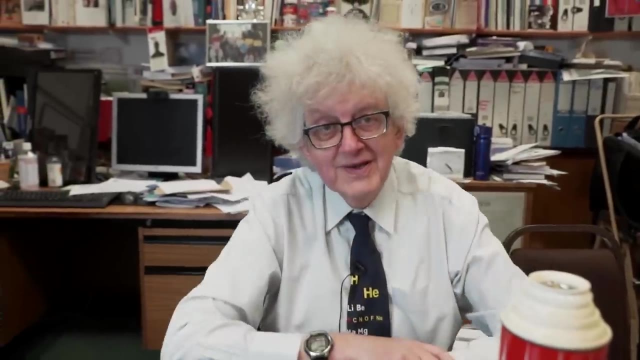 And there was an enormous explosion. All that was left of the thermos was the plastic top and this piece of metal. Everything else was distributed around the lab, But I think the importance of this is to show you that arsenic, If you get it. 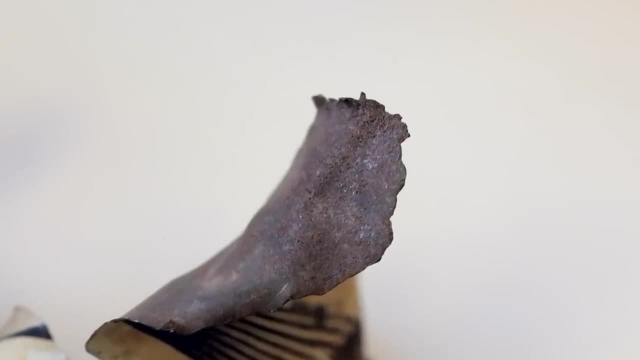 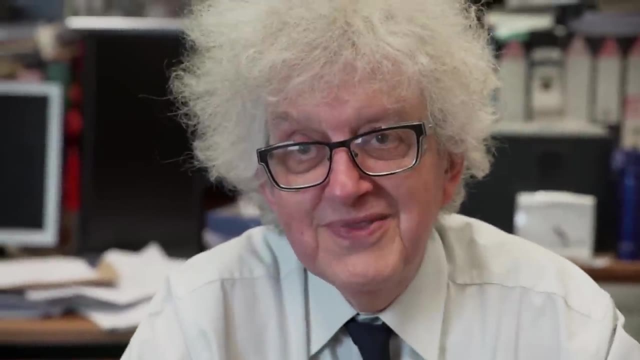 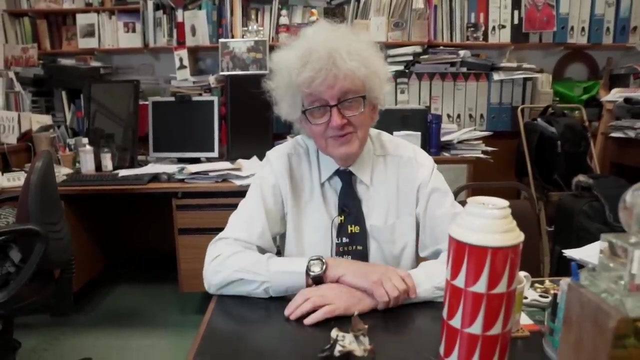 In the right state- or perhaps I should say the wrong state- can react very violently. I went into the lab before it had been cleaned up and retrieved this because I was just so amazed by it, And I used to use it when I was teaching about arsenic chemistry. 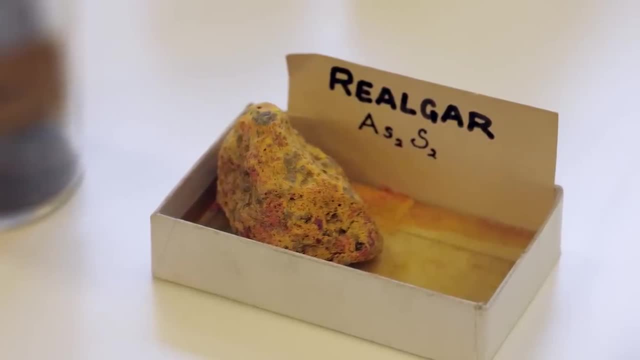 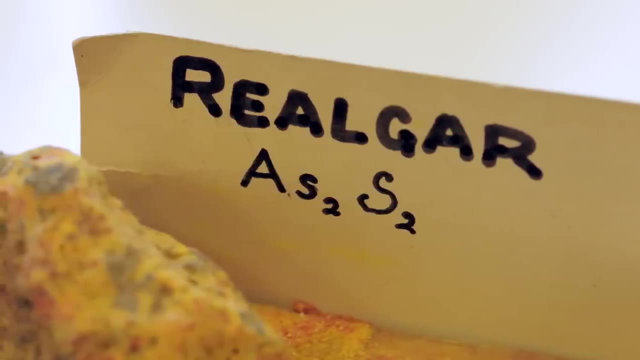 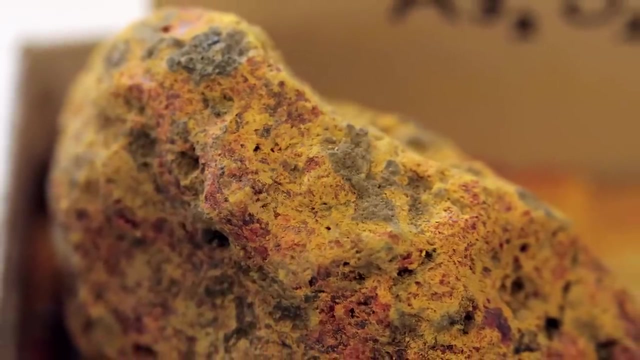 Apparently metallic arsenic can occasionally be found in natural minerals, but usually it's found as compounds, And in our store We have a sample Of minerals containing arsenic that's called Realgar. It's an arsenic sulfide which has really very nice red crystals. 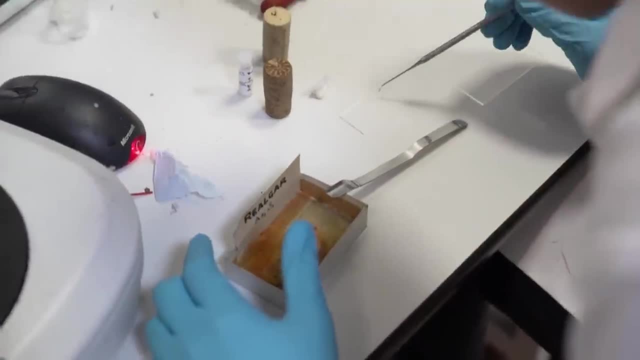 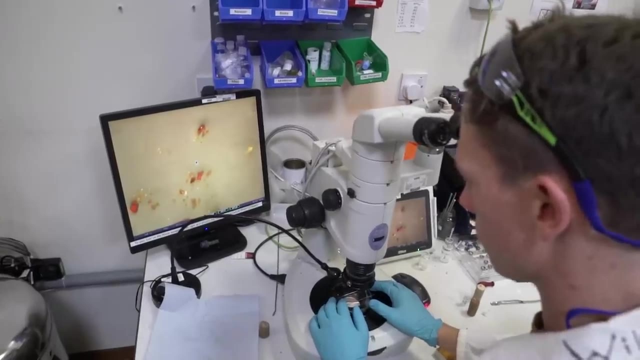 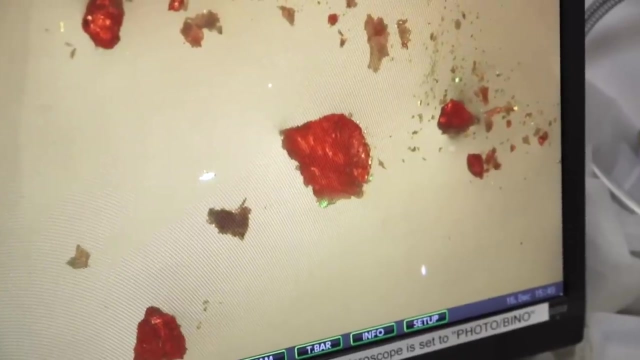 Unfortunately, our sample has rather small crystals, but if you look at them under a microscope you can see really nice red crystals which are of arsenic sulfide, And this is probably why arsenic compounds were known even in ancient times because of these brightly colored minerals. 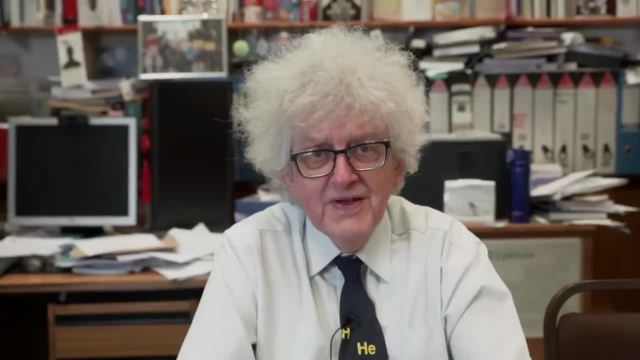 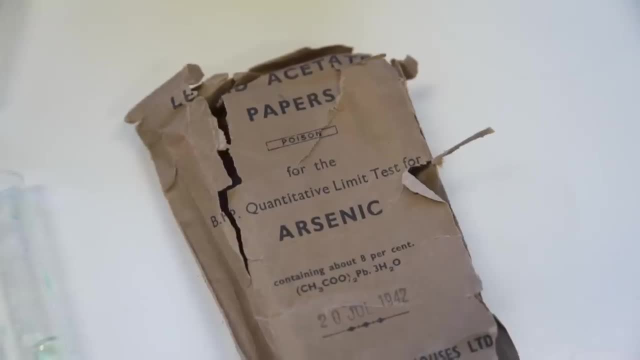 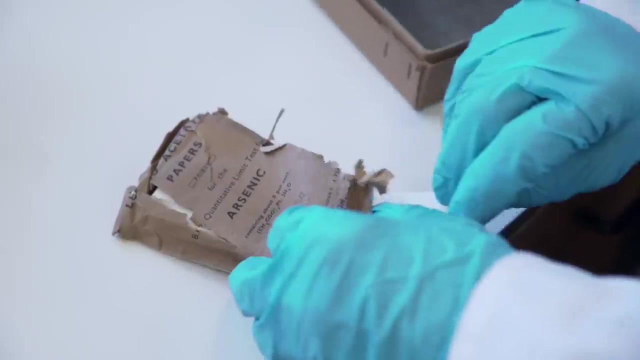 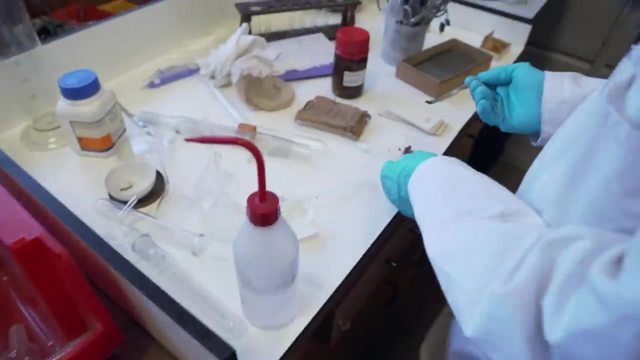 While we were filming, Neil found some amazing old papers- Lead acetate papers- for testing for arsenic. They were labeled 20th of July 1942, before any of us were born. So we tried these papers out. We tried testing them on some of Neil's mixtures that he'd made.